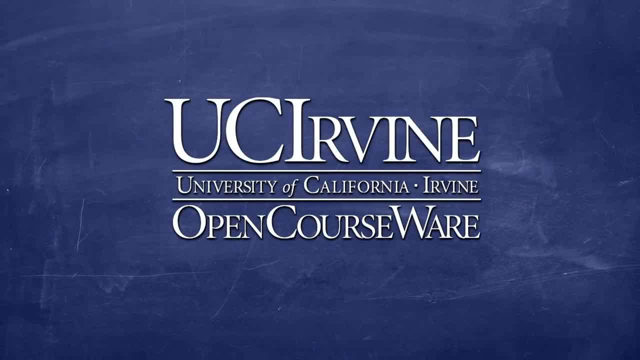 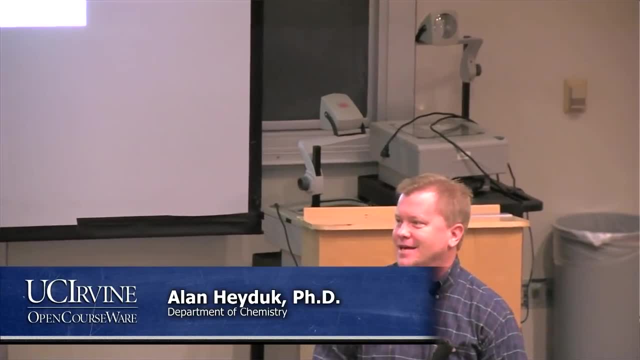 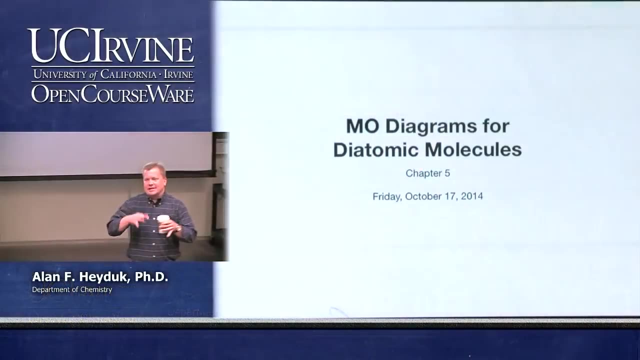 Okay, good morning everybody. Thanks for coming. Oh, that's. I love it when people say: good morning back. See, we're going to change the dynamic here. okay, because I know Matt's kind of like very stiff and proper. I'm not, So the good news is, maybe we'll. 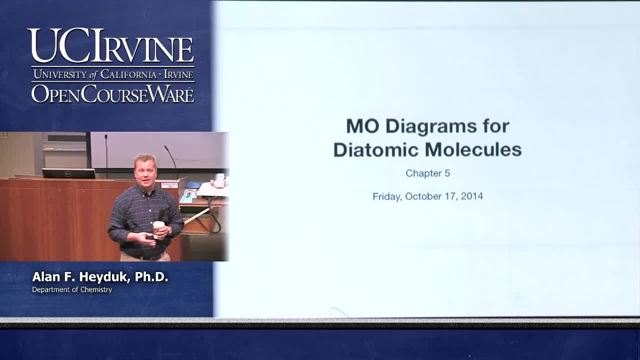 have a little bit of fun. The bad news is, when you go to watch these videos back online, the ones with me are going to be all deleted out. You know it's going to be just one big like beep beep. No, But that's okay, We'll still have fun. So we're going to pick up. 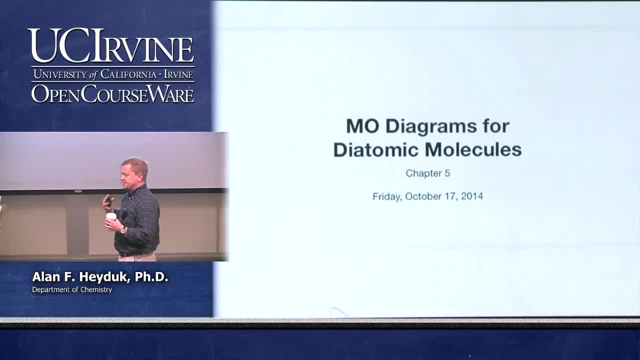 where Matt left off last time, talking about and introducing the concept of molecular orbital theory, We're going to get a little bit more complicated and work up to those diatomic molecules that you learned way back in freshman chemistry. So, yes, we're going to just keep rehashing things that you already know but maybe put 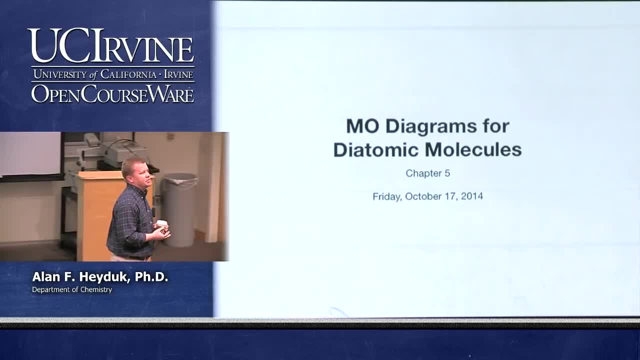 a little bit of a deeper spin on it so that you have a better appreciation for how molecular orbital theory works. And that'll really help you next week when Matt comes back and takes you into larger molecules, And in the second half of the quarter when I take over and 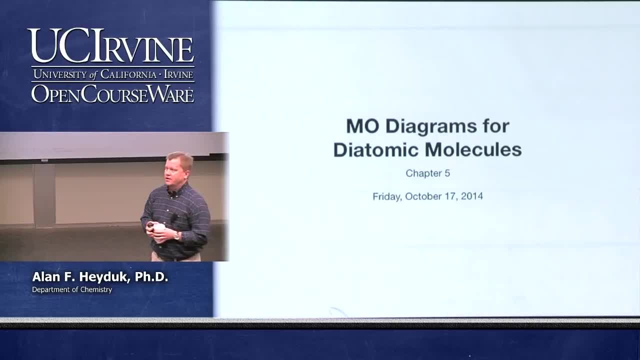 we really start looking at transition metal complexes. things are going to go kind of haywire on the MO theory front. okay, It's going to get a lot more complicated. So it's really, really important that you get a bulletproof understanding of these concepts. 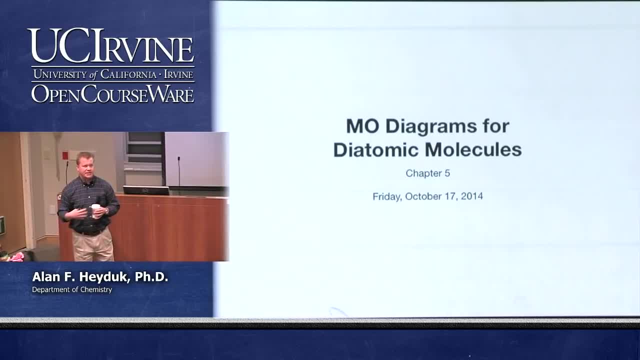 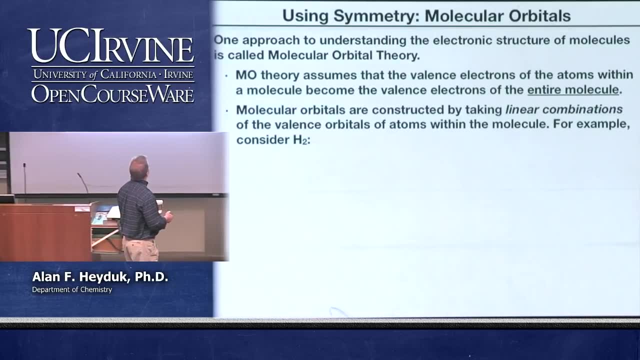 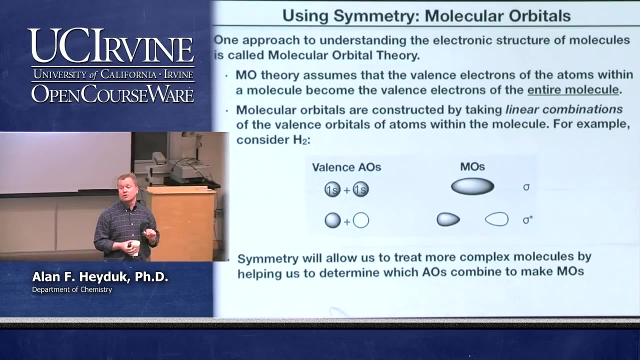 with simple diatomics now, so that when we get to the crazy molecules it's not quite so daunting. So last time- okay, lots of animations here. It's great. Last time Matt introduced the sorry Professor Law introduced the concept of molecular orbital theory to. 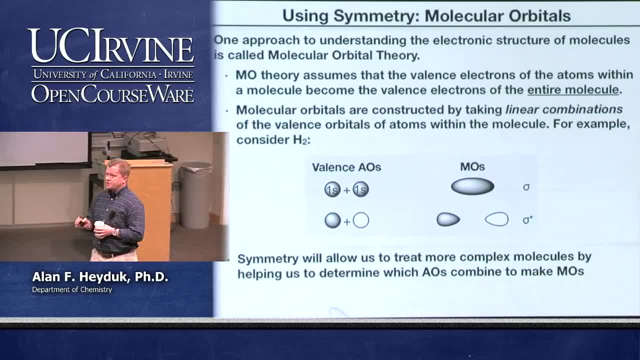 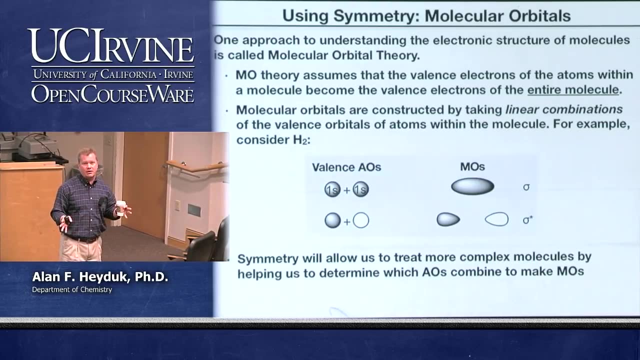 you again. The important thing that I want you guys to always remember is molecular orbital theory is a model that we use to describe the electronic structure of molecules. It's one model. There are many other kinds of models. okay, If you want to think about it. I like analogies. 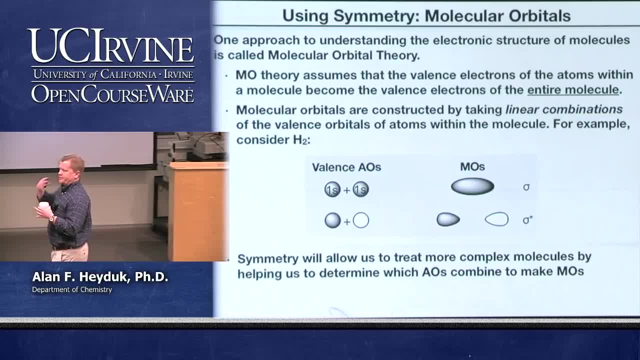 so Legos are one way of building models of cars or spaceships or whatever. okay, You can also go to the store and buy those little plastic models that look like a Fordic model. Mustang, that's a different type of model. okay, each model is a little bit. 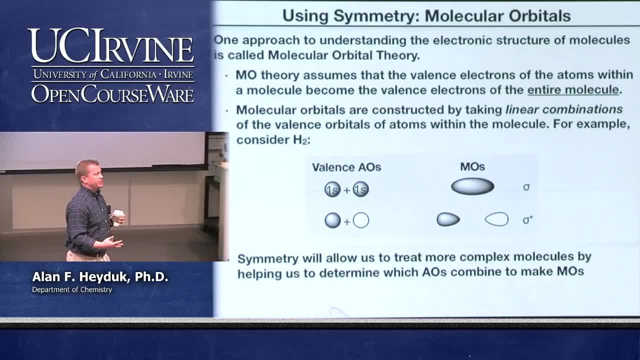 different. it makes different approximations. so mo theory is one type of model that we use to describe the electronic structure of molecules. it's not the exact electronic structure. we're not that smart. okay, that's really what it comes down to. we can solve the exact electronic structure for basically two. 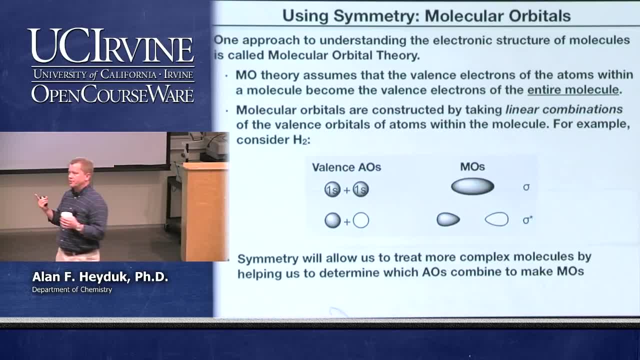 cases the hydrogen atom. okay, we can solve the Schrodinger equation because there's one electron, and we can solve the Schrodinger equation for the h2 cation. so we can put two nuclei and remove one electron and solve the Schrodinger equation again. anything else we can't solve the Schrodinger equation. 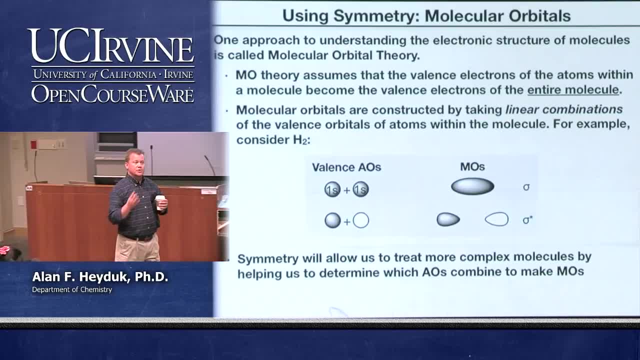 so we come up with these cheesy models to help us approximate. what's great about them is they allow us to understand trends. they often are pretty good until you get to asking really fine detail questions. but mo theory is one model, and now, within that model of mo theory, the specific type of mo theory that we're gonna talk about is: 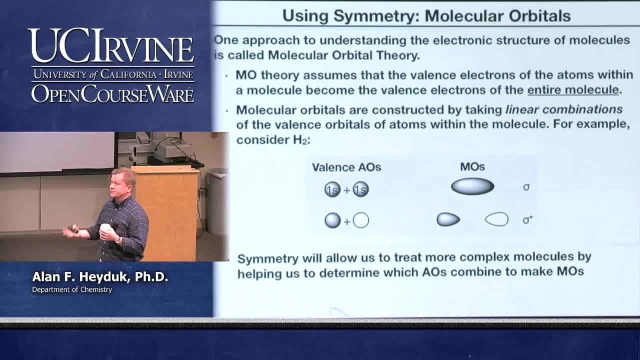 the linear combination of atomic orbitals approach. okay, so when we build our molecular orbitals, we're going to use the atomic orbitals that we're all familiar with: the s orbitals, the p orbitals, the d orbitals. we can all draw these in our sleep, and so it's what we would call an easy basis set, if you want. 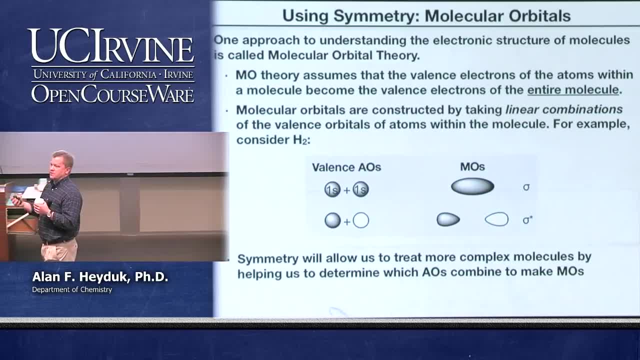 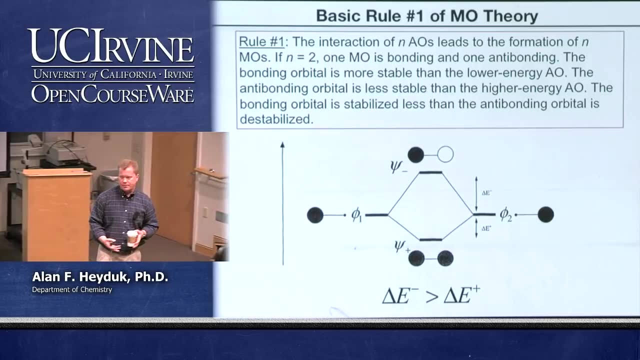 to go back to the Lego model, it's a an easy set of bricks that we all understand to put together to build more complicated structures. Okay, So rule number one when we're doing this linear combination of atomic orbitals approach, as Professor Law introduced last time. 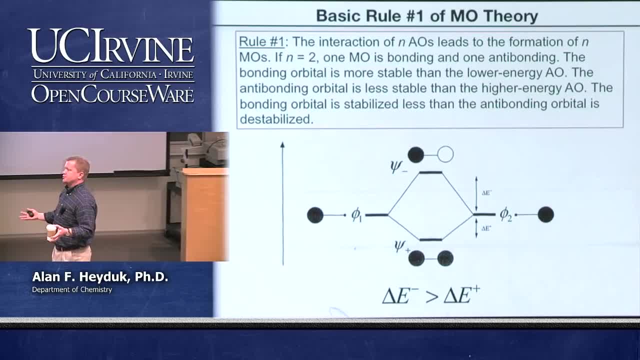 when we say linear combination of atomic orbitals sounds really complicated. It just means we're taking orbitals and adding them together in different combinations. Linear combination means you're adding them together. If you start out with two atomic orbitals, like two S orbitals. 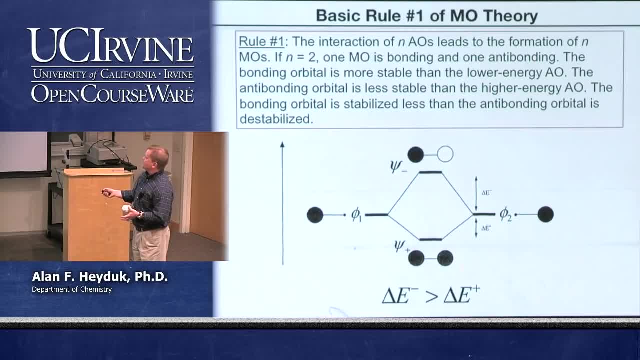 you're going to combine them in a linear fashion and you're going to get two molecular orbitals. In this case, we get the in-phase combination that we saw last time, that we call a sigma bond, And we get the out-of-phase combination. 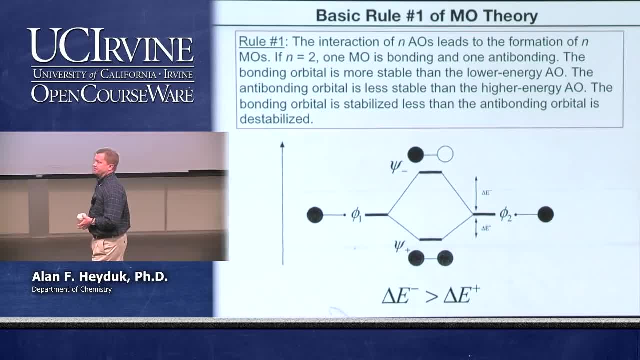 that we call the sigma star or the anti-bonding combination. We saw last time how these are only approximations of the picture. Really, what happens is you get a building up of electron density on this bond, the inter-nuclear separation between the two nuclei. 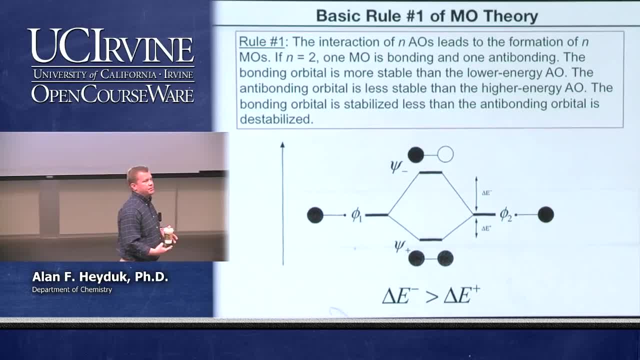 Okay, The reason that we get a buildup of electron density there is because- remember, these orbitals are wave functions. When you add waves together so that they're in phase, they reinforce each other, the amplitude of the wave gets larger, and so that's what we call increasing electron. 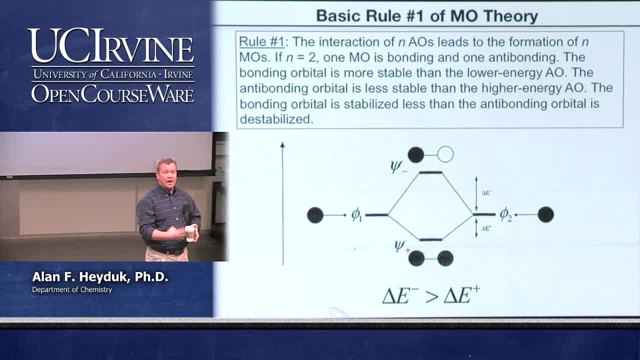 density in between. If you add two waves together and they're out of phase, you get destructive interference. All right, We know a wave right. So if you add a positive wave together with a negative wave, if they're exactly out of phase, they cancel each other out. 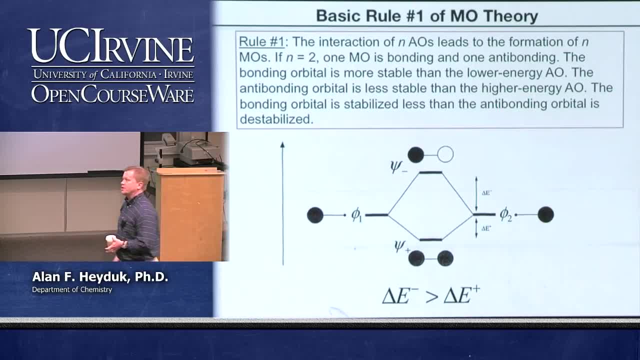 You get destructive interference. You get a node. That's what we call an anti-bonding orbital. There's zero probability of the electron being in between the two nuclei. Okay, The math. Professor Law went through it a little bit last time. 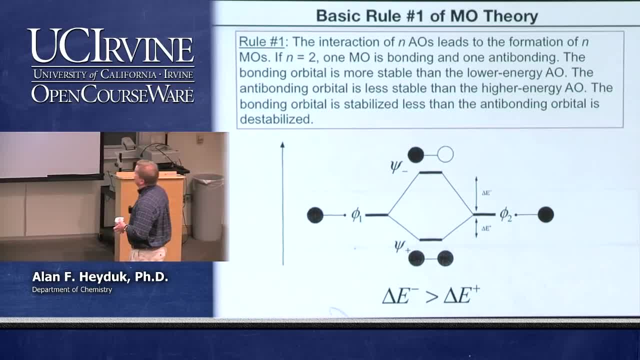 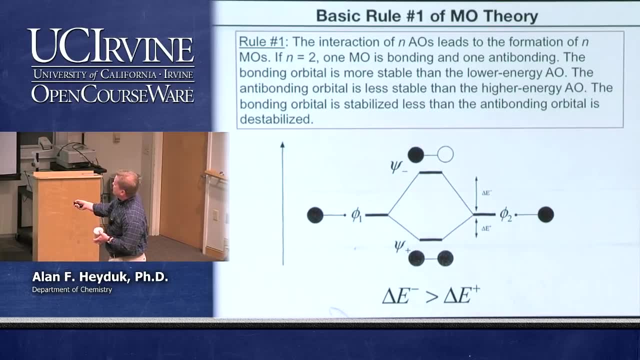 I have trouble calling him Professor Law, He's just Matt to me. So the bonding orbital. Matt went through the math a little bit. that describes this. the bonding orbital gets stabilized by less energy than the anti-bonding orbital, gets destabilized. 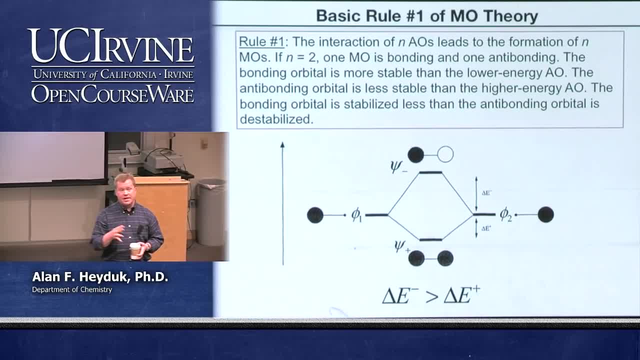 That's always true, though in a lot of molecular orbital diagrams you'll lose that information just because they get complicated and it's hard to draw it in. but you always have to remember that this bonding orbital is stabilized by less than the anti-bonding orbital is destabilized. 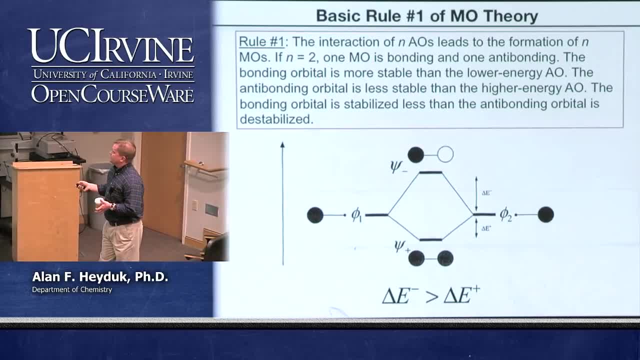 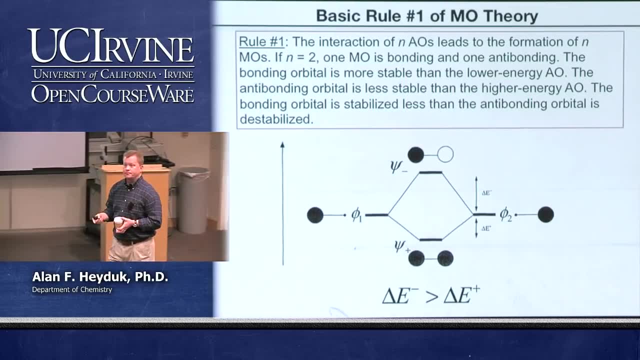 There's another consequence that was touched on briefly Last time. the bonding orbital is always smaller than the anti-bonding orbital. The anti-bonding orbital is always bigger and more diffuse than the bonding orbital, And both the energy effect and the size effect come. 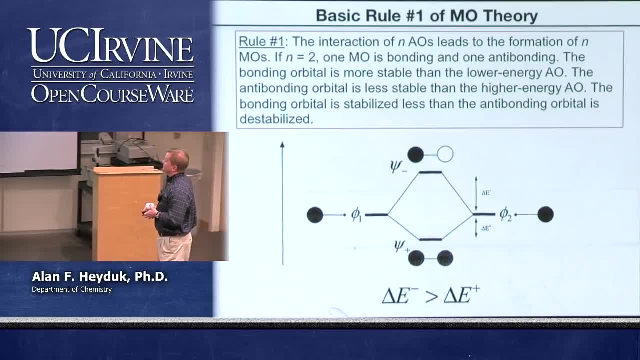 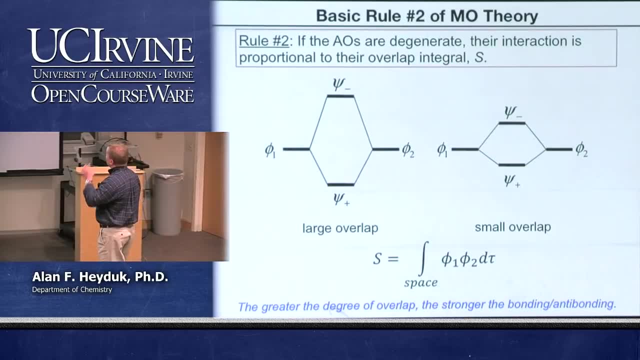 out of the overlap integral, that S squared term that was introduced last time when Matt went through the math. Okay, So rule number two: If the atomic orbitals are degenerate, their interaction is proportional to the overlap integral S. Okay, 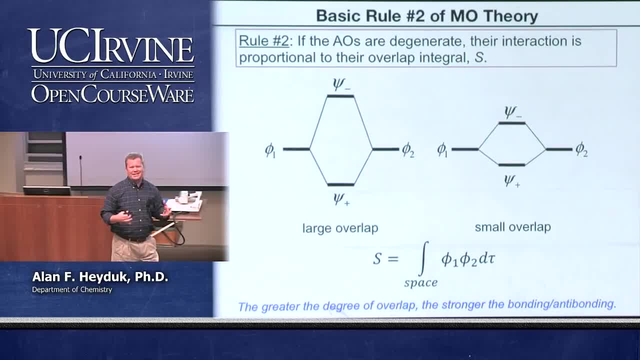 Now again, qualitatively. this should just make sense to you. If we were to have a hydrogen atom over here and a hydrogen atom over here and we said how strong is the bond between them? You'd say pretty darn weak. 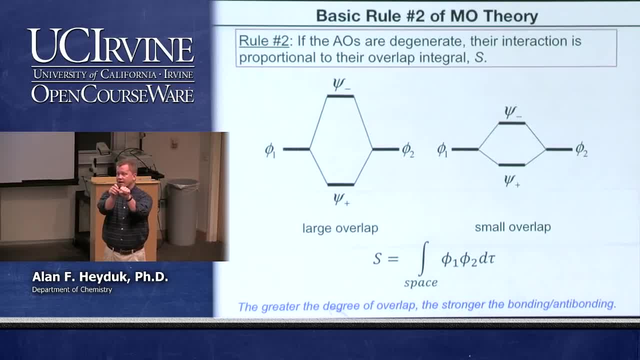 They're too far apart. But if we bring them right next to each other, at the distance that two hydrogen atoms form a bond, 0.8 angstroms. well now, all of a sudden, the orbitals are in close contact. 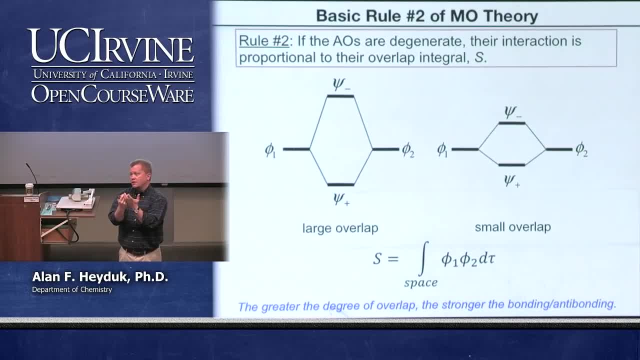 You get a good overlap and the bond becomes strong. Okay, Again, this is like I said. I like analogies. It's like long distance relationships, right, If you're going to have a long distance relationship, you're going to have a long distance relationship. If you're close together, it's easy to you know it's a strong bond, everything's great, You know. if you're far apart, well okay. We know how long distance relationships usually work out. That bond becomes weak. 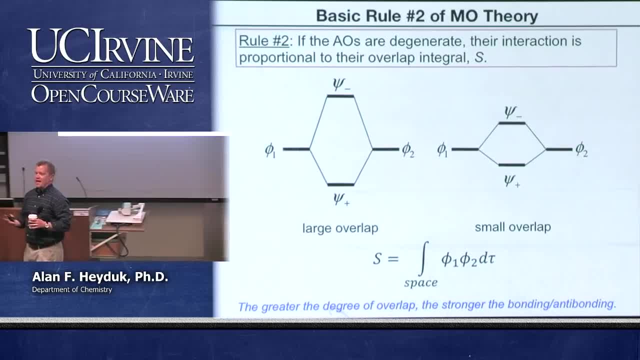 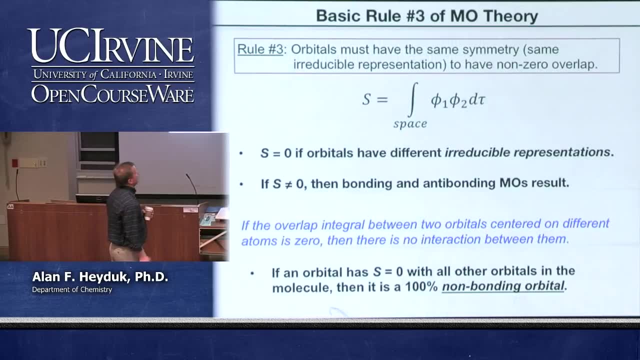 All kinds of other things cause problems, But it's the overlap integral. The closer these orbitals are together, the stronger the interaction is going to be. So, really, what we're doing there is we're solving this sophisticated integral that relies on two wave functions. 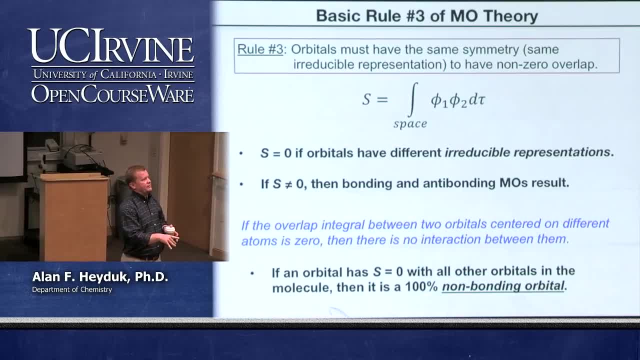 that you've seen the equations for before And if you ever tried to do something with them, they gave you nightmares. At least, they give me nightmares trying to do the integrals and everything. That's why we like symmetry, So we spent all that time teaching you point groups. 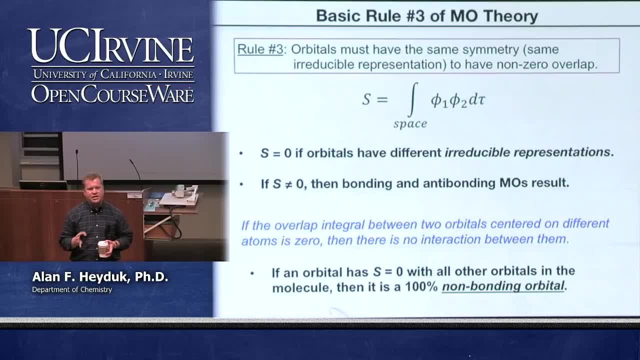 and symmetry operations because group theory gives us the incredible power To predict when the overlap integral is exactly zero. That's really the whole point of why we did symmetry, Because you can now predict when the overlap integral between two orbitals is zero without actually solving the integral. 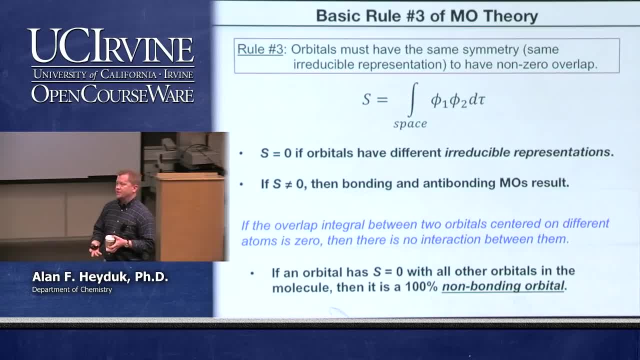 without actually looking at the wave function for the orbitals and doing all kinds of crazy math. If the two orbitals belong to the same irreducible representation S is not zero. If they belong to different, irreducible representations S is zero all the time. 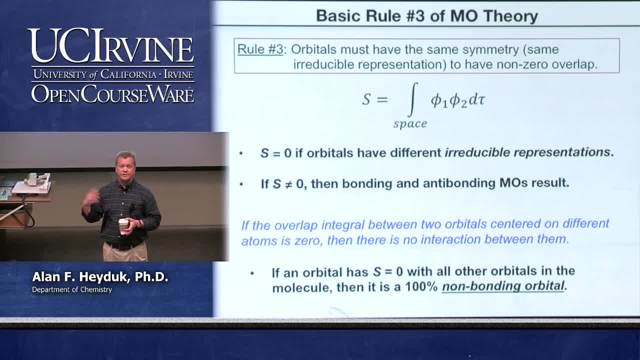 You can't form bonds between orbitals that are parts of different irreducible representations. It's fantastic, It doesn't OK, I'll be honest with you. It doesn't really matter that much for diatomics, because you know more or less. we're talking about eight orbitals. 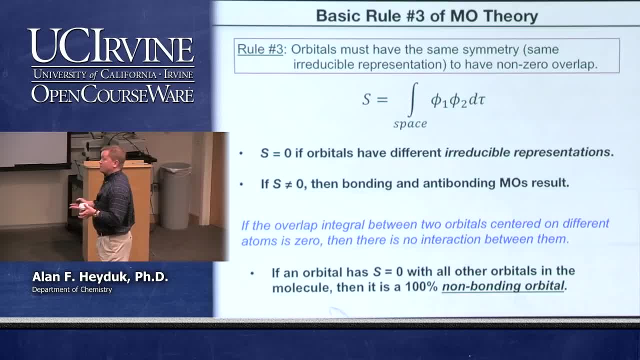 You can figure it out faster than you can do the symmetry, But when you're talking about something like a porphyrin molecule and there's 25 atoms and each atom brings at least four orbitals, and you're trying to sort all these things out, 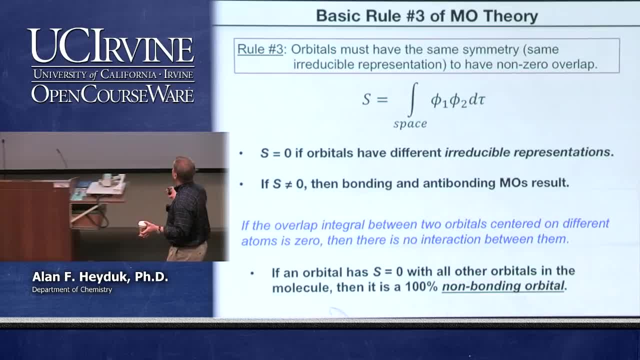 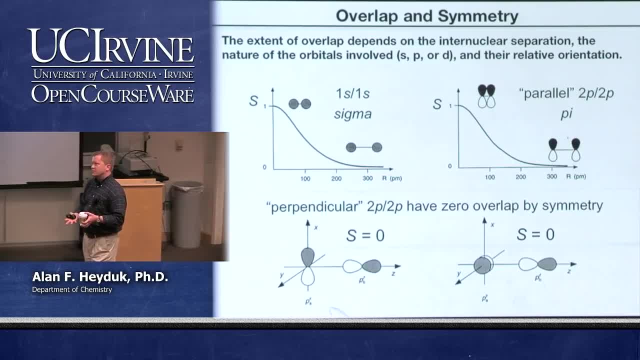 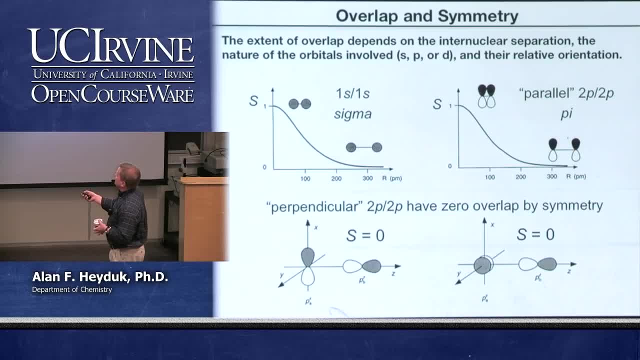 Here's. so I actually don't like these graphs because they, on the x-axis you have the internuclear separation and on the y-axis you have the overlap integral, And so you can see they start here at zero. Well, if you have an internuclear distance of zero, 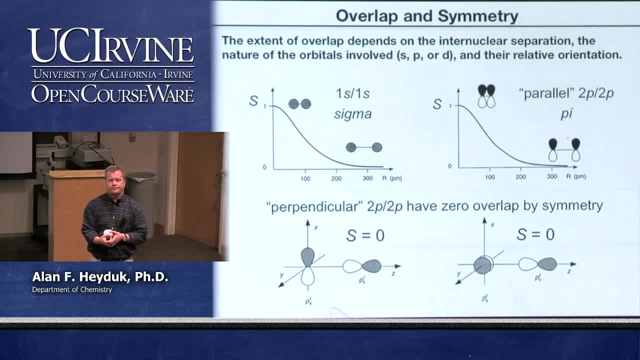 then that means the two nuclei are right on top of each other. Well, this is showing you that the overlap integral, that's the highest. That should be the best right. Clearly, if the overlap integral is one, you're getting perfect overlap. What's the problem? Two, Yeah right, Two positively charged nuclei are not going to want to be in the same spot. Okay, So you never get a diatomic. you never get a diatomic. you never get a diatomic. 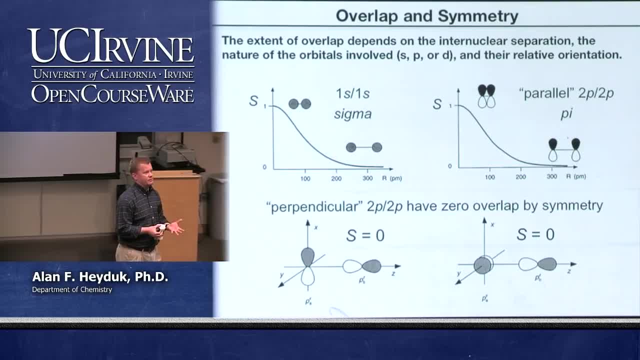 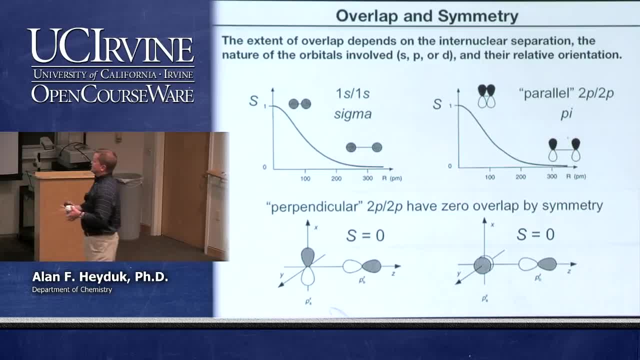 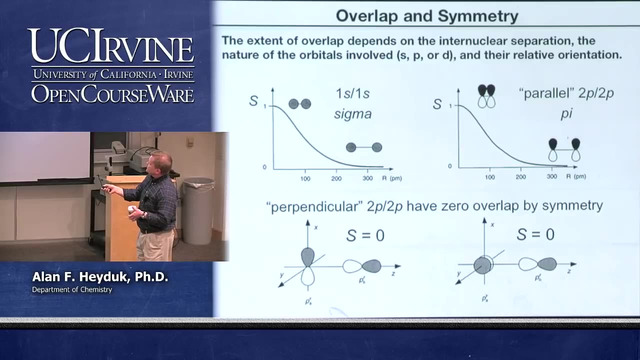 So while it is true that the overlap integral maximizes at a distance of zero, it's not a realistic picture of what the bonding surface looks like. Same thing happens with two parallel pi orbitals, But then here we can see, on the bottom half, these two pictures. 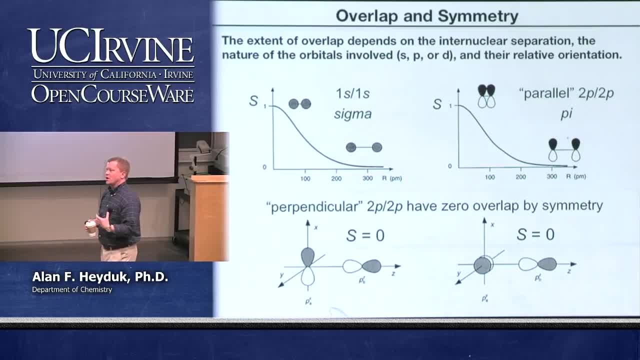 show us what happens, What happens when we have orbitals that belong to different representations. Okay, If we were to go through and do the symmetry on a diatomic molecule, we would find that this: I guess this is the px orbital and this is the pz orbital. 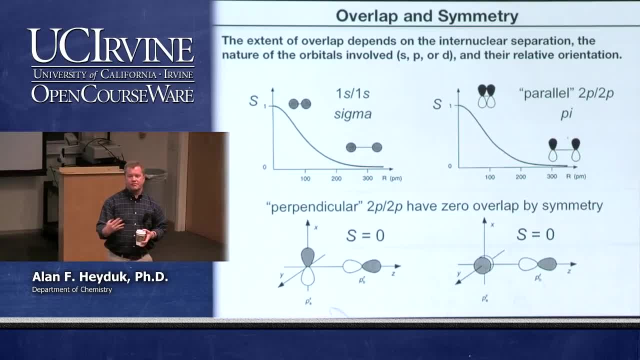 Okay For a diatomic molecule. those will always be parts of different representations. We know, because they're different irreducible representations. the overlap integral is zero. Pictorially we can look at it. we can say, okay, this is unshaded, it's going to interact in a positive way here. 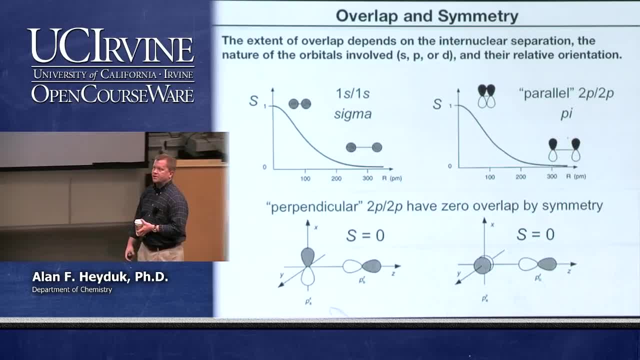 and in a negative way there it's going to cancel out. Okay, So you can do it with pictures. you can do it with this rule number three: You can solve the integral if you're, you know, one of these overachiever types. 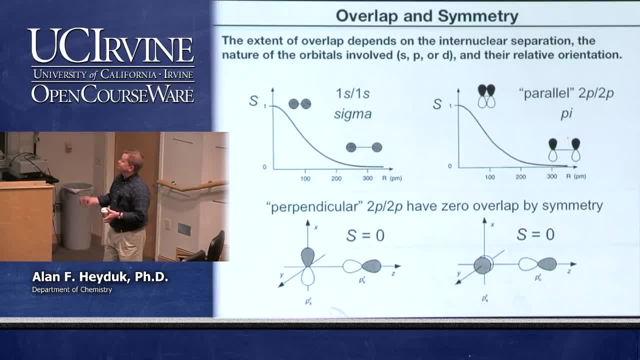 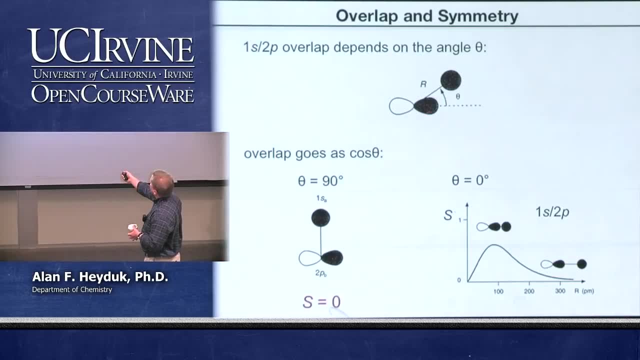 That's never been me, so I like cartoons. Okay, Same thing here when we're talking about the overlap integral. There are going to be cases and we're going to- you're going to get into these next week and we'll really get into them later. 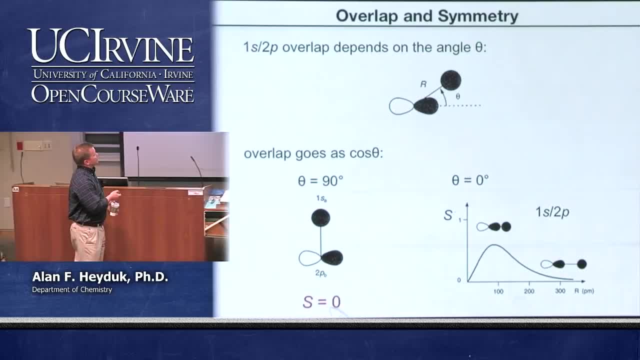 in the quarter when we deal with transition metal complexes where it's not exactly clear cut how the two orbitals are interacting. So you can see, in this case we have an s orbital coming in at an angle that's less than 90 degrees to this p orbital. 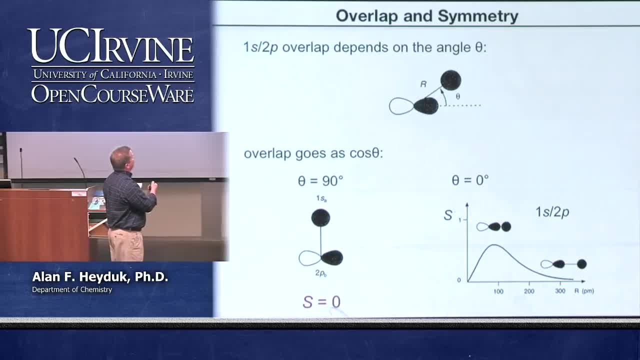 Okay, This is a p orbital. This is a special case, It's not. you can't get it with a diatomic. Okay, We'll see it with molecules that are threefold symmetric, and so on, But in this case you get a positive interaction. 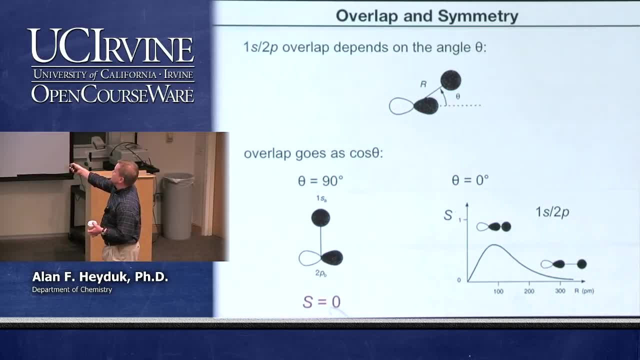 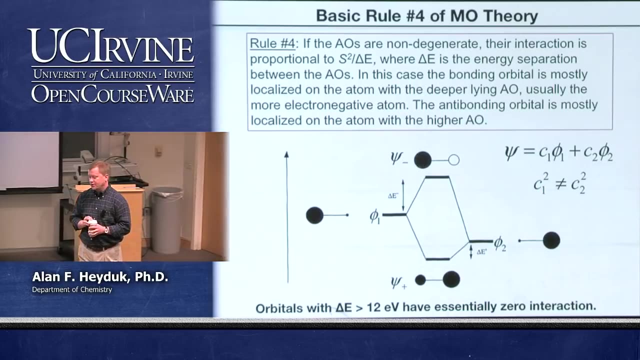 You form a sigma bond, because this shaded s orbital interacts with this shaded lobe of the p orbital Much more strongly than it does with that unshaded orbital. Oh sorry, That was rule three. Okay, Last one, rule four. 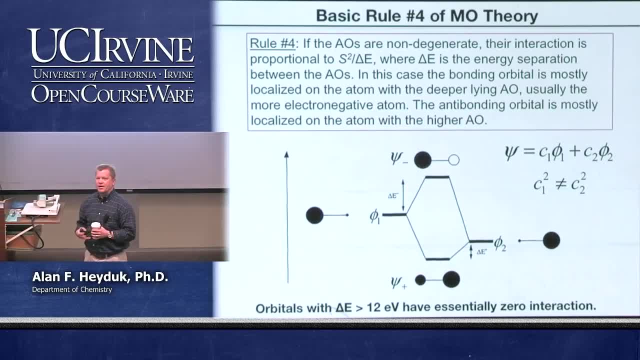 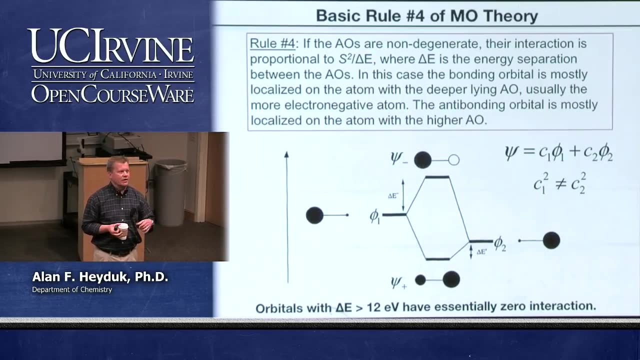 Rule four deals with the interaction between non-degenerate orbitals. Point of vocabulary. when we talk about degenerate in quantum mechanics we mean they're the same energy. Okay, I know there's some- you know- colloquial meanings of the word degenerate, but we're not talking about that. 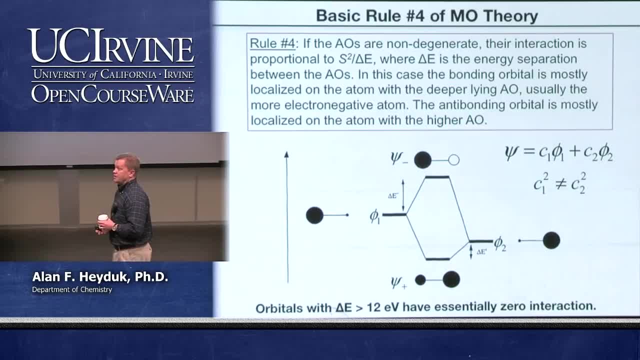 Definition. Okay, Degenerate means the same energy, So when we talk about non-degenerate orbitals, we're just talking about two orbitals that have different energies, For instance, a carbon 2p orbital interacting with an oxygen 2p orbital. 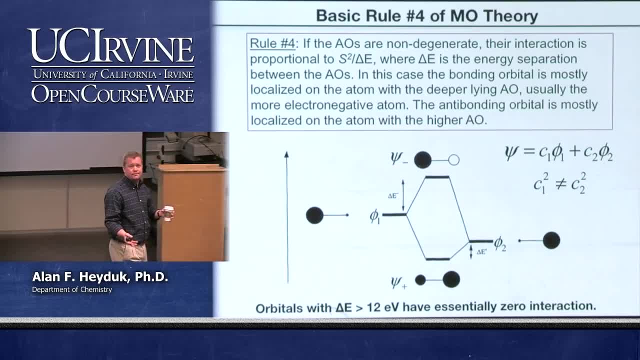 We know that carbon and oxygen have different electronegativities. Electronegativities reflect the energy of the valence orbitals. Therefore they must be at different. you know the orbitals must be at different energies. That's going to impact the strength of their interaction. 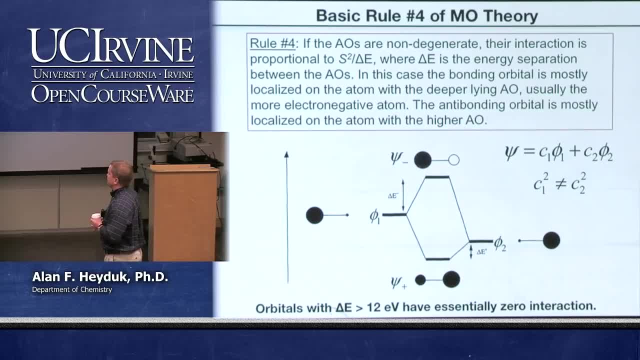 And so what we can see here? this is just done with two s orbitals. not two s orbitals, but two s orbitals. Right. In this case, the s orbital on atom one is higher in energy than the s orbital on atom two. 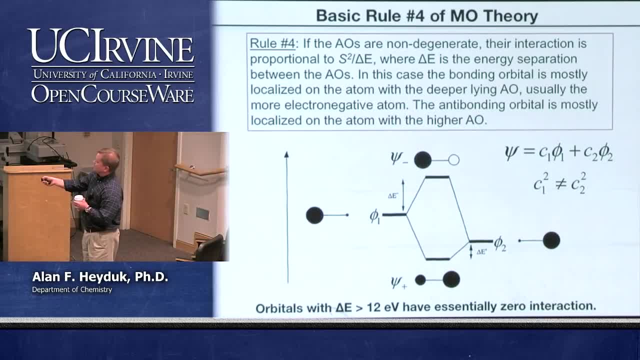 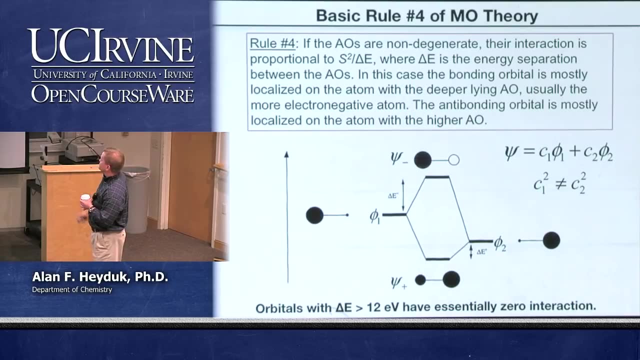 We represent that by remembering that energy is always going to be plotted on the y axis. so we write this orbital higher in energy. The bonding combination still is stabilized Right. It's lower in energy than the lowest atomic orbital. The anti-bonding orbital is higher in energy. 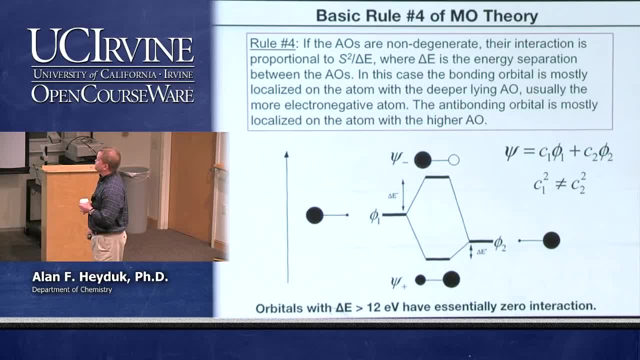 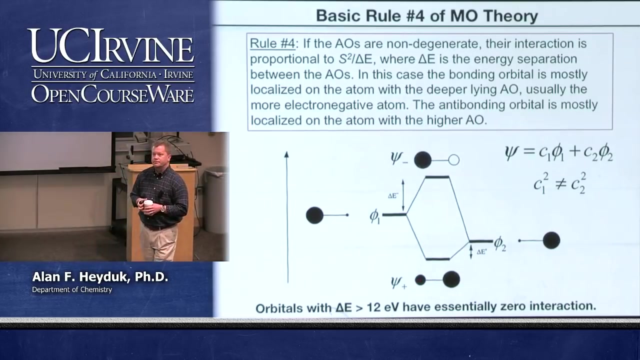 than the highest atomic energy atomic orbital. You'll notice another thing happens, or is represented by these cartoons: The bonds polarized right. If we look at this bonding orbital, we have unequal sizes for the two circles. This is how molecular orbital theory deals with polarization. 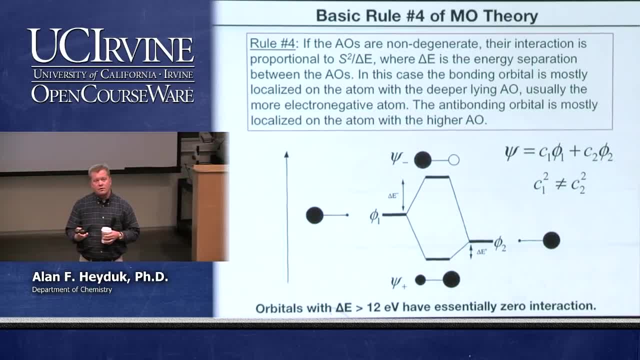 Right, We know that if we take a hydrogen atom and we bond it to a fluorine atom to make HF, the electrons are all going to be polarized to the fluorine side. Right, We all know how to assign dipoles. 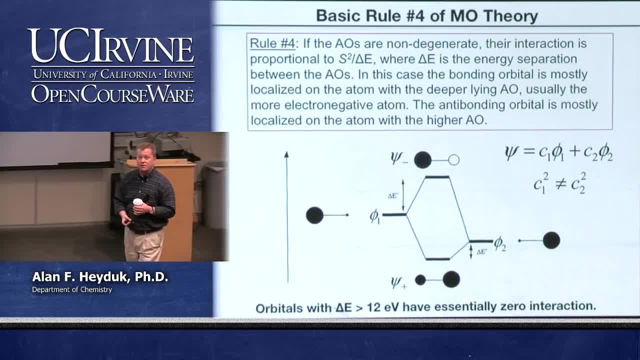 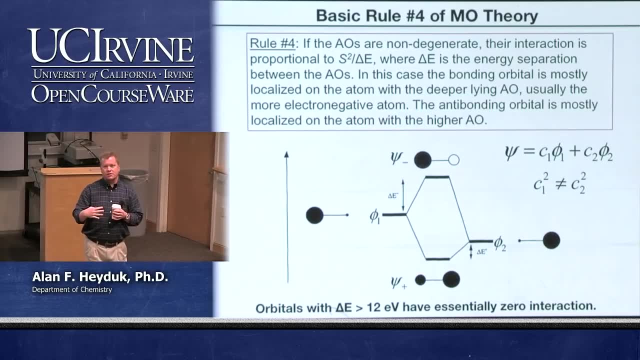 Well, this is how we describe it in molecular orbital speak. The bonding orbital gets localized on the lower energy atom or the atom that contributes the lower energy orbital. The anti-bonding orbital gets localized to the lower energy atom. The bonding orbital gets polarized to the atom. 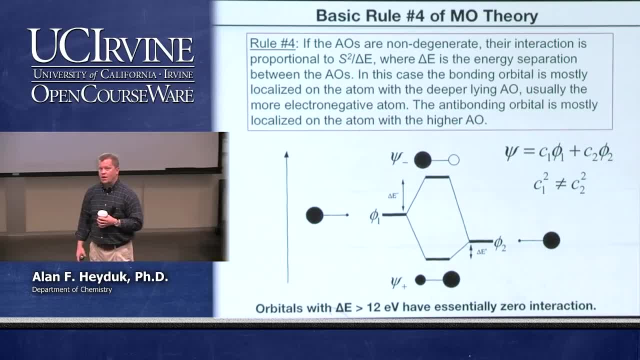 with the higher energy orbital. So now, if you are having flashbacks to 51, you could assign different names. Right, Atom 2 is going to be the nucleophile side. Atom 1 is going to be the electrophilic side. 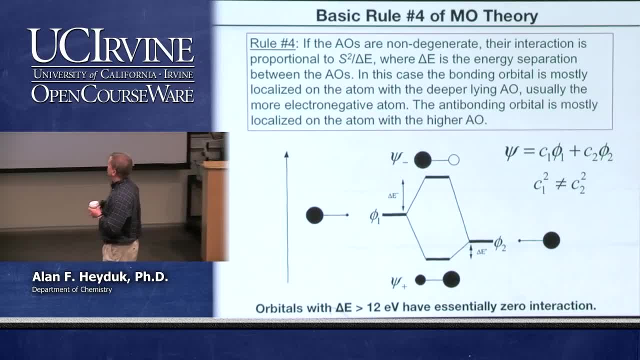 Right. So we can't do that Right. This anti-bonding orbital is going to be the Lewis, acidic or electrophilic side of the molecule, So there's something interesting down here. Orbitals with a difference in energy greater than 12 EV. 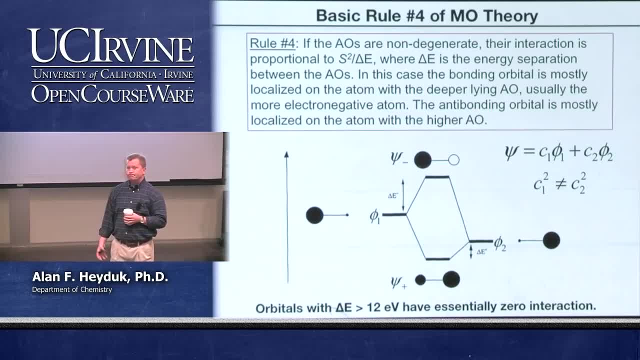 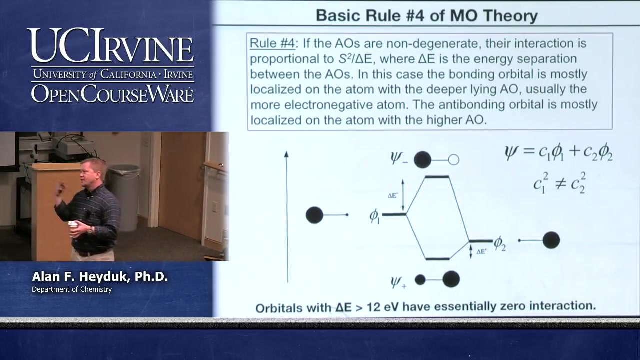 which is huge, okay, have essentially no interaction. That seems kind of weird. So I don't have all the numbers of the periodic table memorized, but and there isn't even a periodic table in this room, Fantastic. But let's, we know, okay. we know HF, we know lithium fluoride. 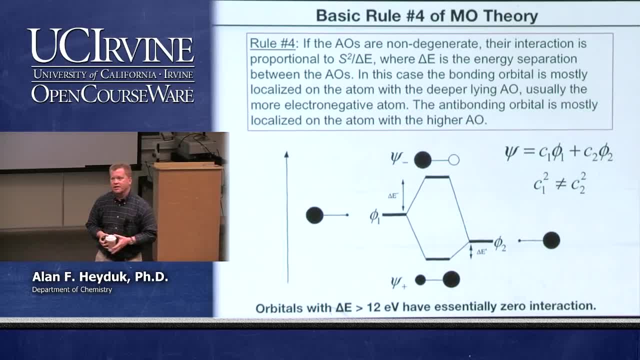 Let's drop down one of the last elements in the first column on the periodic table is rubidium. It's one of the most electropositive elements on the periodic table. We know fluorine is one of the most electronegative. 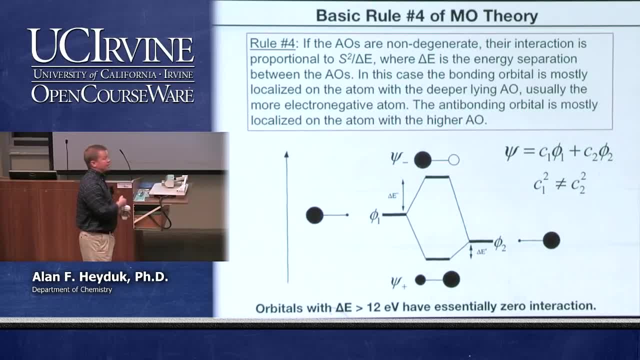 So let's assume that they're. the delta E between the orbitals on rubidium and on fluorine are zero. Do you think rubidium fluoride exists? That's salt. It does. You can make rubidium, It's a salt. 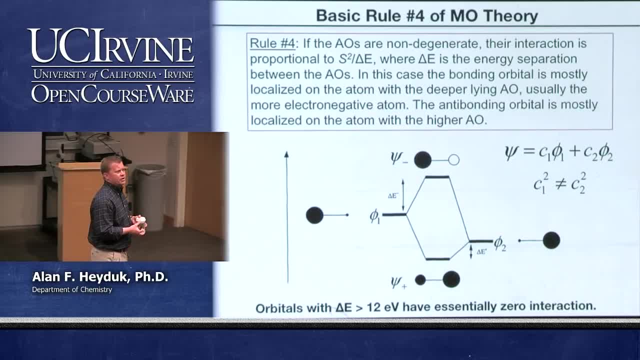 Solid at room temperature. So how does rubidium fluoride exist if we're telling you that there's zero interaction between the orbitals? Oh, ionic bonding. So remember when I told you MO theory was just a model. When you have models, 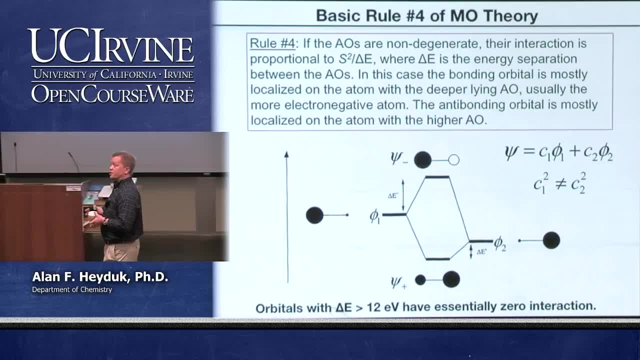 you make assumptions. If you try and apply your model to a system where your assumptions aren't valid, your model's a piece of junk. If you're talking about something like rubidium fluoride or lithium fluoride or anything in ionic salt, MO theory is not the way that you want to describe it. 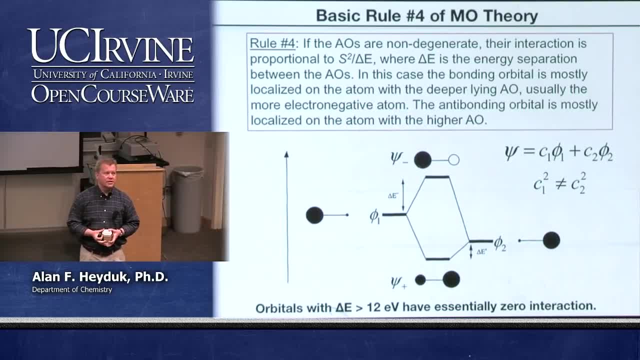 because this bonding model was really developed to describe covalent. Well, this is called covalency, not ionic bonding. So you can still make molecules or compounds or salts when there's a big energy difference. You just can't use MO theory. 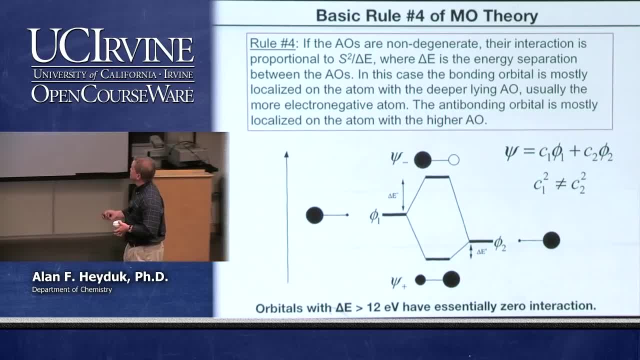 to accurately describe their electronic structure. So the complicated part ends up in that gray area, okay, where you have Fairly large differences in delta E, but the compounds aren't quite ionic. That's where we get the polar covalent bond. 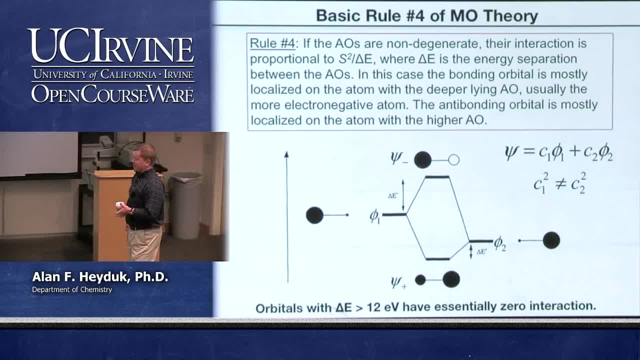 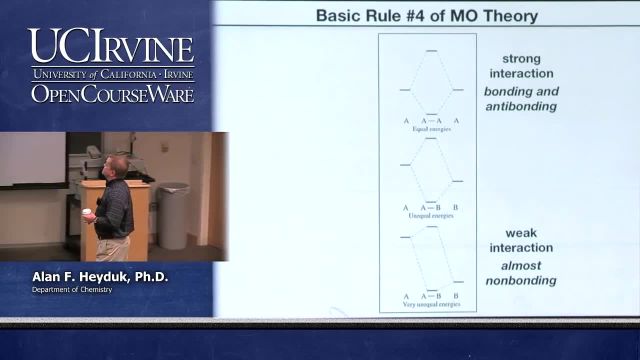 and we describe the orbitals in this way, so that they're polarized towards the more electronegative atom. And so here's three cases. The top case is one where we have the degenerate interaction: Two atomic orbitals of the same energy interacting to form a 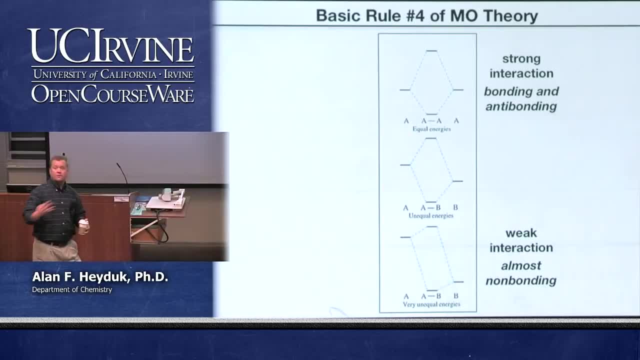 sigma and sigma star. From a covalency perspective, that's when you get the strongest interaction. The strongest covalent bond occurs between two atomic orbitals of the same energy. We know that. We know that a carbon-carbon single bond is stronger. 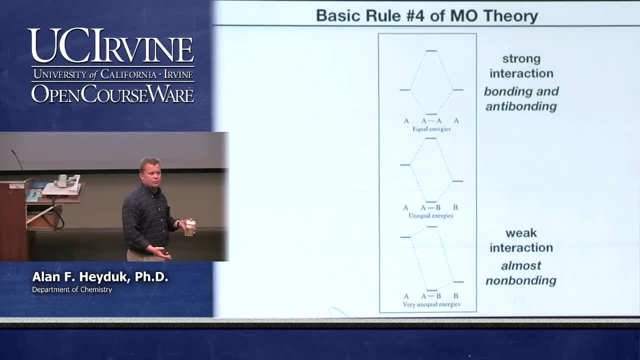 than other carbon-nitrogen bonds or whatever, because it's a covalent bond and the orbital is covalent. The covalent bonds and the covalent orbitals are perfectly matched If we have unequal energies, but they're close. you still get a strong interaction. The bonding orbital will be localized on the lower energy atom, the anti-bonding orbital on the higher energy atom. This splitting between the bonding and anti-bonding is a little bit less than it is in the perfectly covalent case. 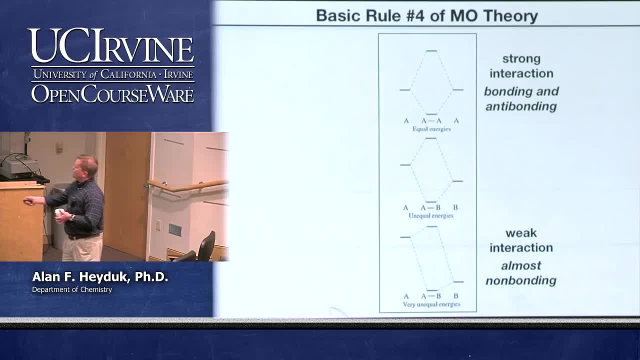 When we get to very high energy, when we get to very unequal energies, what we end up seeing is that this bonding orbital only gets stabilized by a very small amount relative to the pure atomic orbital. This is also going to be the most polarized case. 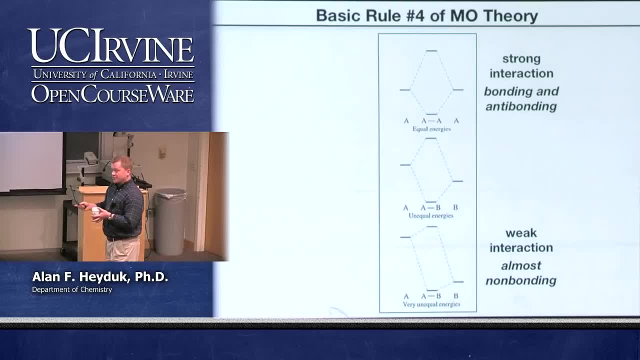 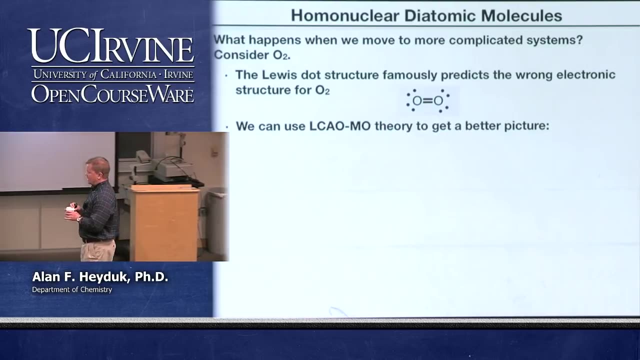 The bigger this difference in energy, the bigger the polarization of the bond towards one atom or the other. Okay, Okay, So those are your rules. Now let's actually get in and make some molecules using more than just S orbitals. So O2 is the classic case. 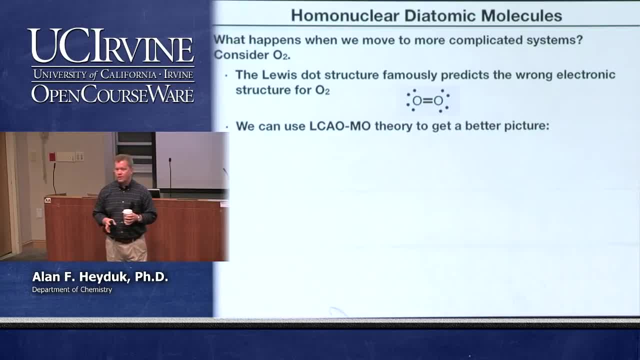 for why molecular orbital theory rocks. okay, Because if you use those you know really simplistic models that they teach you in Chem 51, Lewis dot structures and all this stuff, you get the wrong electronic structure. And if you can't predict the electronic structure, 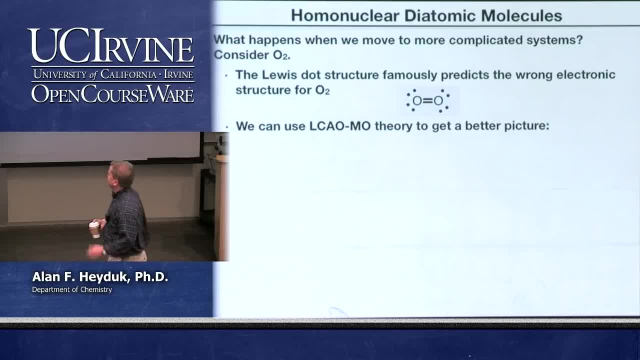 for a diatomic molecule. well, I'm just kidding It. actually, if you do it right it actually does work. But this is kind of the simple dummies guide to Lewis structures that you would get for a, you know, for O2.. 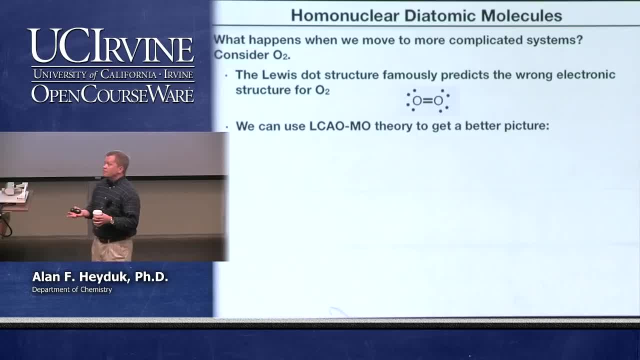 You predict a double bond, which is correct, but you predict that all of the unpaired electrons are paired up And you can do a really, really cool experiment with liquid oxygen. pour it through the poles of a magnet and the magnetic field will bend the stream of liquid oxygen. 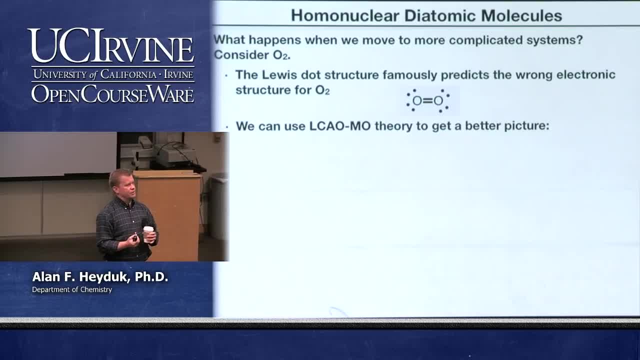 because oxygen has unpaired electrons. It's also blue in color. Okay, Okay, Okay, It's blue in color. Has anybody ever seen these like the oxygen experiments? They're really cool. Plus, if you have liquid oxygen and you drop a match into it. 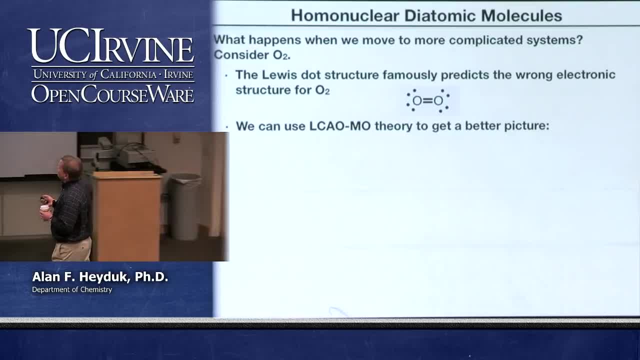 it's really spectacular. So, okay, Lewis, dot structures, don't get oxygen, right? I'm going to let you in on a secret. Okay, How many of you guys are like organic chemists? I can see you wearing a sweatshirt, so 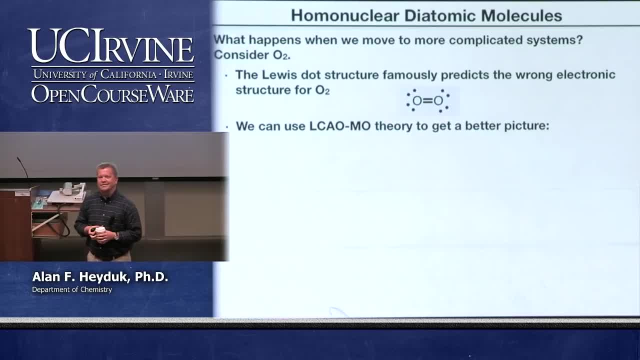 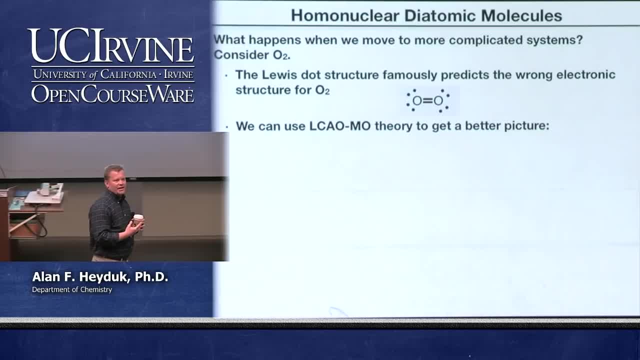 Okay, Okay, The SO. Oh, you know the bonding models they talk about in organic sp two, sp three, hybridization, all that It doesn't even get methane right. I just want you. I'm just throwing that out there. 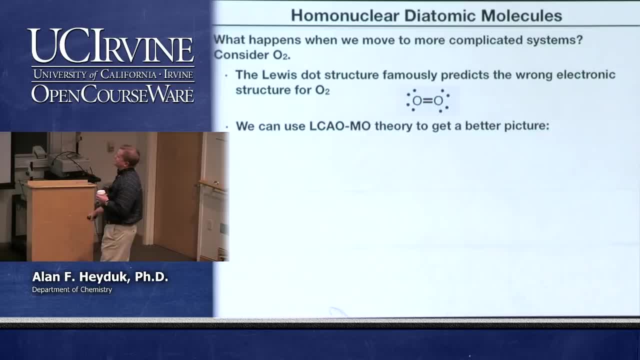 mo theory does Okay. So we're going to use this linear combination of atomic orbitals, molecular orbital theory, to see if we get a better electronic picture of the oxygen molecule. I have a real complex one. it comes to organic chemists. 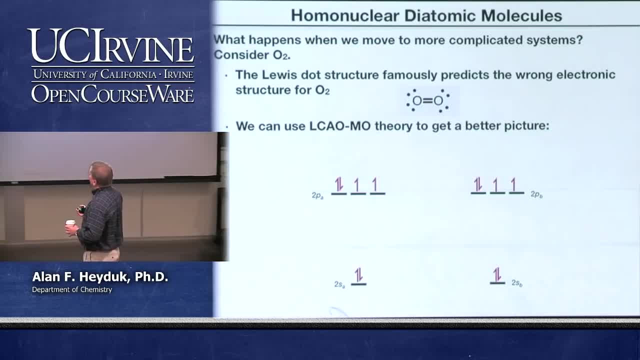 They're smarter than me, so you know I always try and make fun of them. OK, So we know that we're dealing with oxygen. Oxygen is in the second row of the periodic table. It's a p-block element. We count up the number of valence electrons. 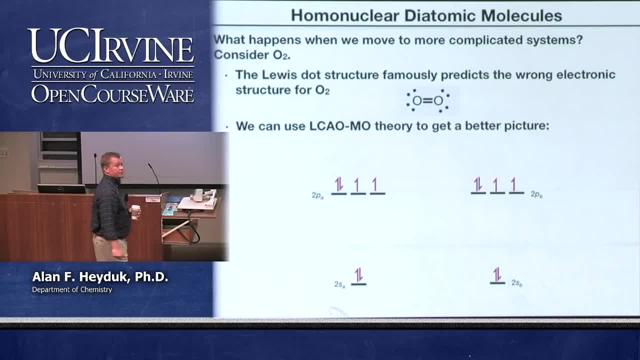 There's six, And so we know that the 2s orbital is lower in energy than the 2p orbital. For oxygen atom A, we put two electrons in the 2s, the other four in the 2p. Same thing for oxygen atom B, Because it's two oxygen atoms. 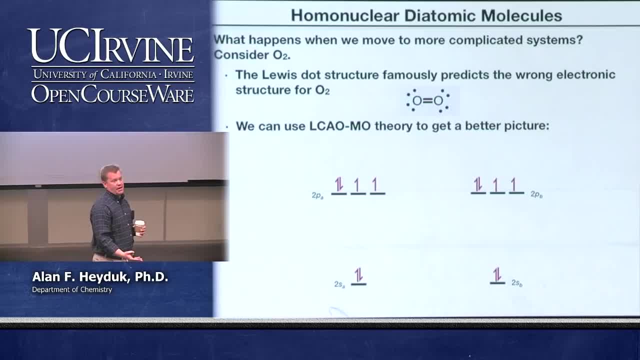 the s and the p orbitals on each atom are at exactly the same energy. This is a degenerate interaction And so now we can go through and we can build up the bonding and anti-bonding and whatever else types of orbitals based on what we know about the shapes. 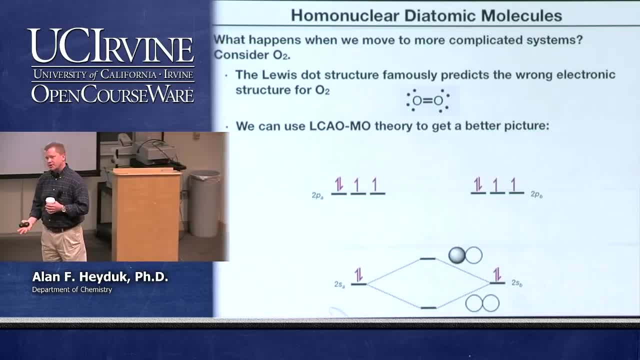 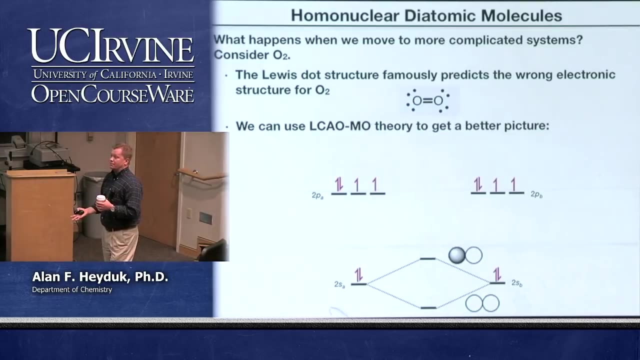 of these orbitals. Now We can use symmetry- OK, But again as easy as character tables are to use for something like dioxygen, where you're talking about the 2s orbitals and a total of 6p orbitals. 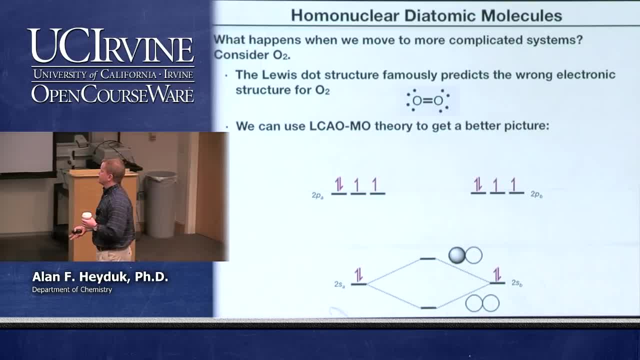 I'm pretty sure you can draw the cartoons faster than you can use the character table. So we take the s. We know that we're going to take linear combinations, So we do an in-phase combination of the 2s's to make a bonding orbital, an out-of-phase combination. 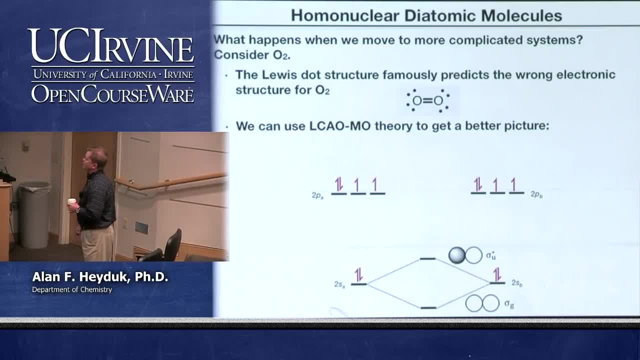 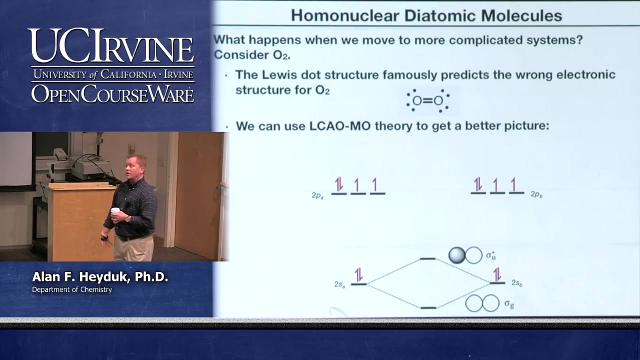 to make the anti-bonding, And then we use a bonding orbital. We can label these as sigma g and sigma star u or sigma u star, whichever order you prefer. This one is g because a homonuclear diatomic has an inversion center. 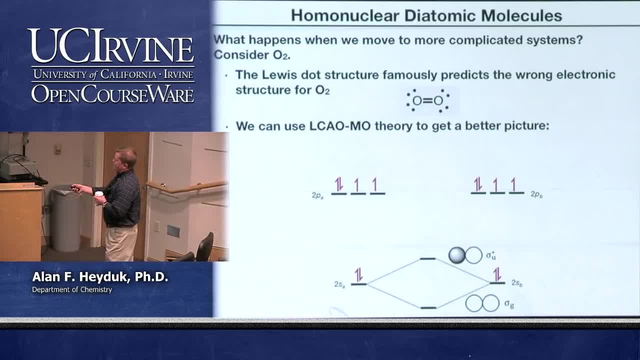 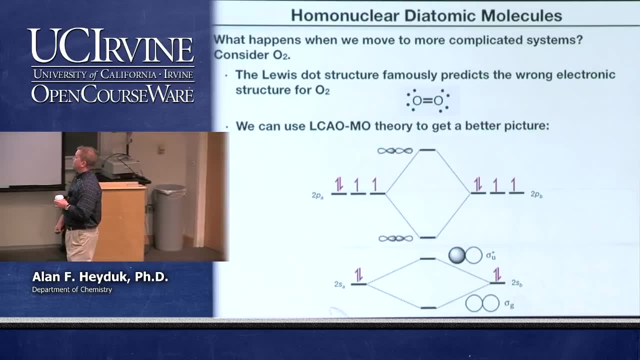 Because it has an inversion center. we can label this as a Garada orbital because it's symmetric with respect to one side. The Ungerade orbital is unsymmetric with respect to inversion. We can make a sigma bond and a sigma star antibonding orbital out of the p-z orbitals. 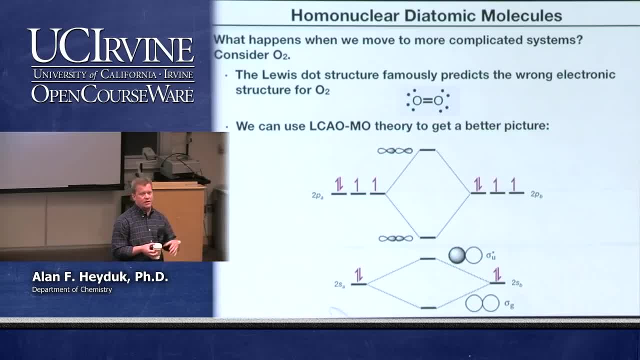 By convention we put the z-axis along the bond, So when the two lobes are shaded the same way, facing each other, for these p-z's you get the sigma orbital- Again, it's Gerada. When they're out of phase, it's sigma star and it's Ungerade. 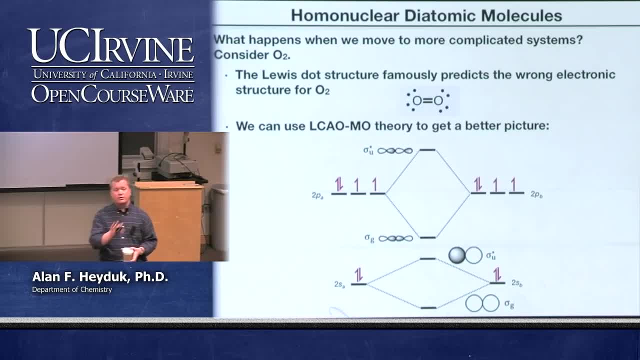 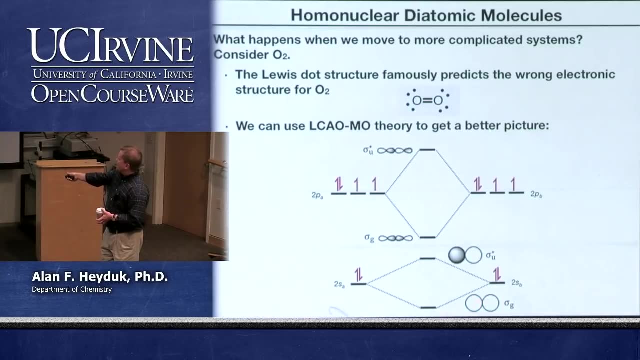 Interesting point here, and this is where you have to be careful When you're being rigorous and you're writing out your equations. remember we're talking. these are linear combinations. This bonding combination Between the s orbitals, we would say, is 2sA plus 2sB. 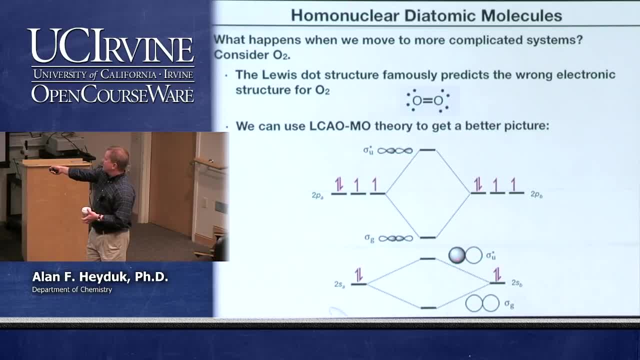 They're added together. This one, we would say, is minus 2sA, plus 2sB. just by keeping the convention the same, You might want to think that any time you add the orbitals together in a positive way, you get a bonding orbital and in a negative way you get an. 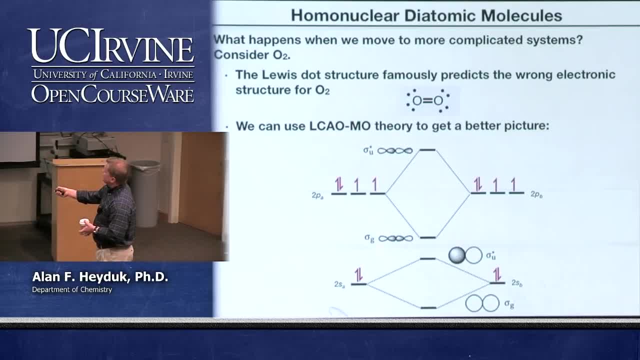 antibonding orbital. That's not true, though. In this case you'll notice that the phasing on the left p-z is opposite of the phasing on the right p-z. This is really 2pa minus 2pb, whereas the antibonding orbital is 2pa plus 2pb. on the 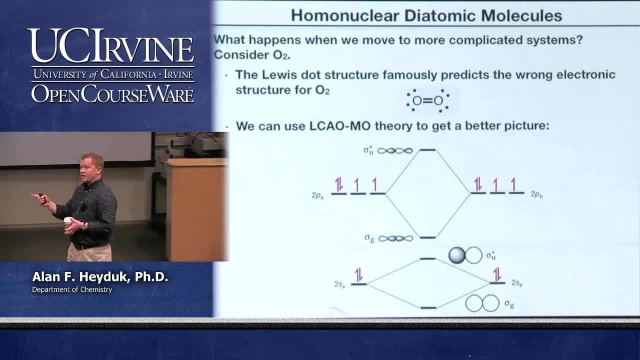 z-axis. The plus and the minus doesn't tell you necessarily that it's a bonding or antibonding orbital. You have to draw out the shading to make sure you are getting it right. There's the sigma manifold. We still have two orbitals left over on each atom. 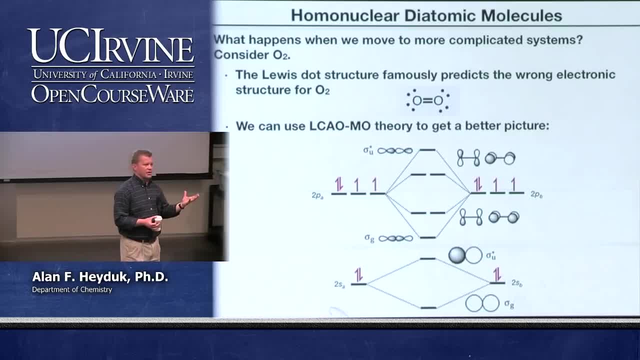 It would be the px and the py. Of course, we know how to draw these. It's the pi bonds. It's the pi bonds, It's the oxygen atoms. These two are in the plane of the board, These two are coming out at you. 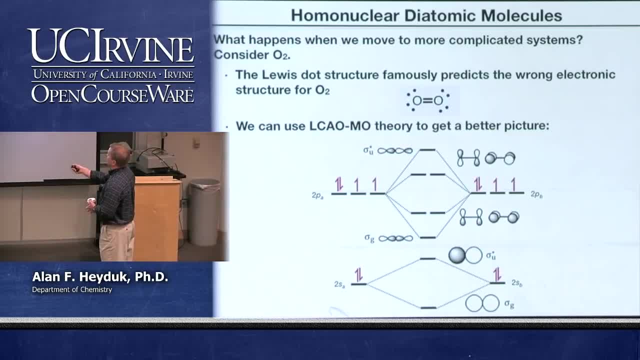 The shading on the lobes matches. These are the pi ungarata because, again, if you put an inversion center at the middle of that OO bond, it's unsymmetric with respect to inversion. The antibonding, or pi star, is now garata. 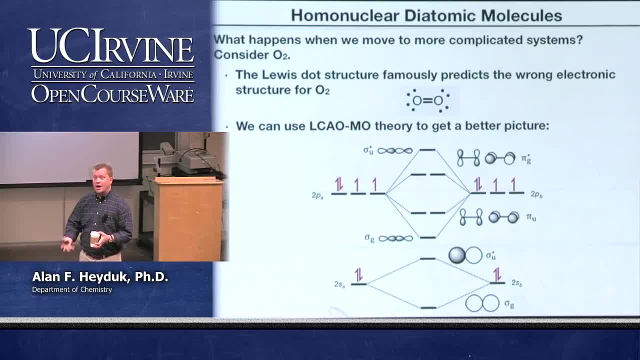 Again, Just because an orbital is garata doesn't mean it's bonding. Just because it's ungarata doesn't mean it's antibonding. You have to look at the actual orbital and decide, because ungarata can be bonding or 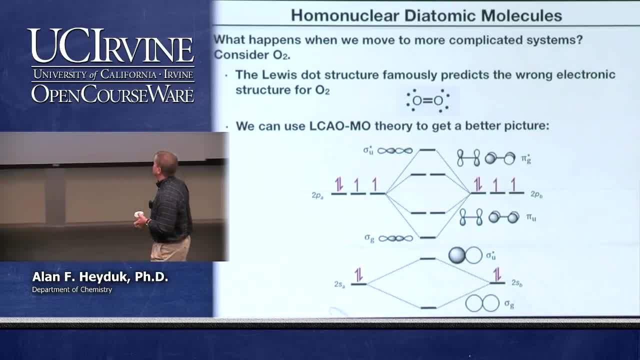 antibonding. It just depends on the actual shape of the orbital. Okay, We now have 12 electrons to put in. We fill from bottom to top. for now We're always going to fill in in lower energy orbitals before we fill put any electrons. 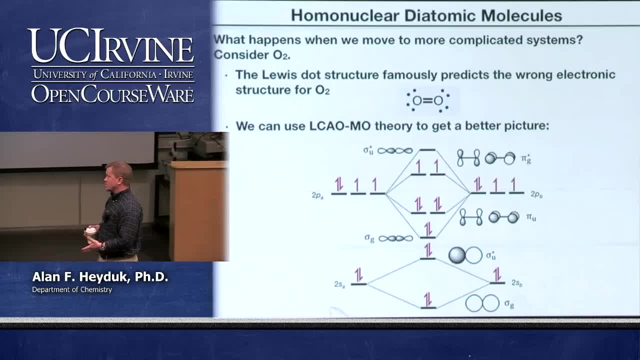 in a higher energy orbital That will change later in the quarter, just to make things confusing. So we get 10 electrons in these two orbitals derived from the S's, the sigma derived from PZ, the pi's derived from PX and PY, and that leaves us two electrons to go. 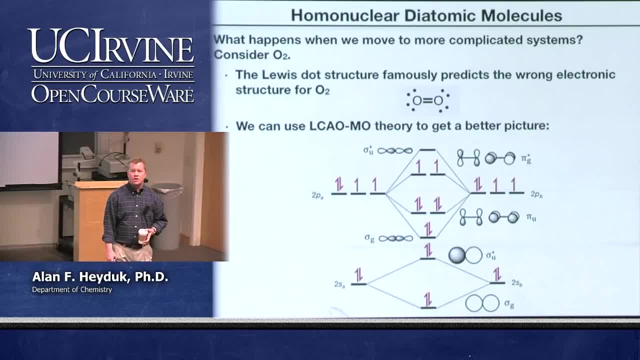 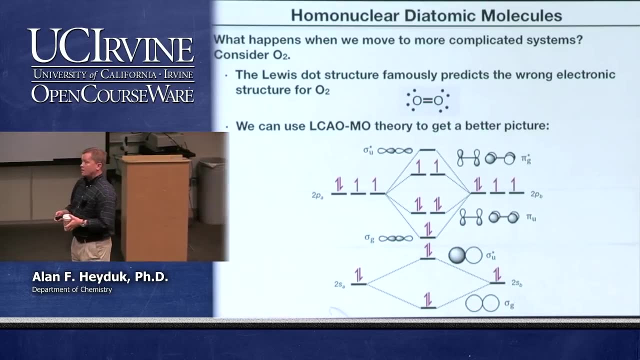 into the pi star orbital. So bingo, right away we predict that O2 is paramagnetic. It's got two unpaired electrons in the pi star orbitals. The other thing that happens when you populate an anti-bonding orbital is: 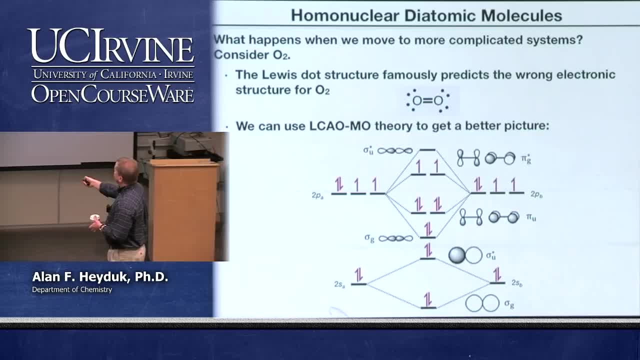 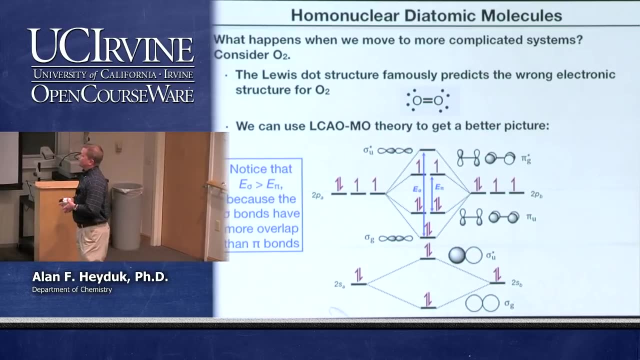 of course you break down the bond order. So, based on this, we have four electrons in the pi bond, but we have to subtract. We've tracked out the occupancy of the anti-bond, which drops the bond order. You can see there's two different energies. 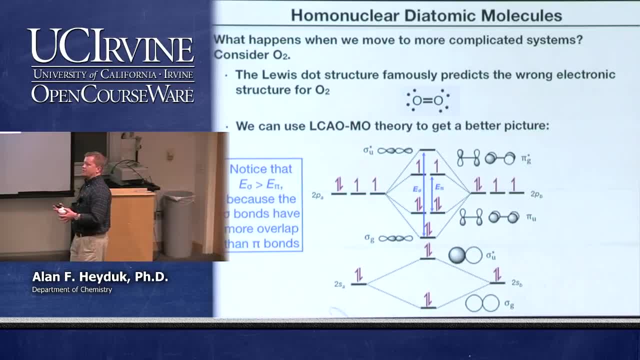 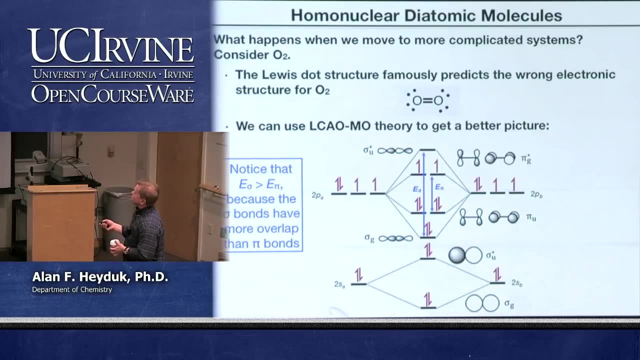 different splittings depending on whether you have a sigma bond or a pi bond Right, All of the P orbitals start out at the same energy. That is an approximation that we may come back to later. But if we assume that all the P orbitals start, 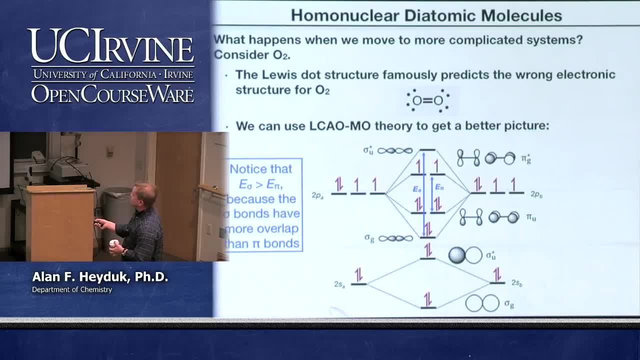 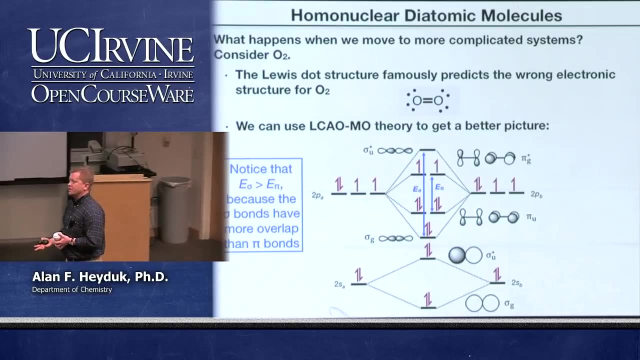 out at the same energy. the sigma interaction is strong, so that sigma bonding orbital comes way down much further than the pi bonding orbital. Again, this is exactly in line with what you learned in organic chemistry in Chem 51. Sigma bonds are always stronger than pi bonds significantly. 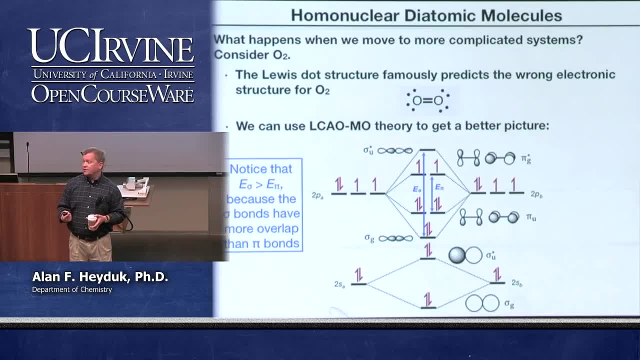 OK, And it goes back to rule number three or two or four, whatever rule it was right. Why is it? why is a sigma bond stronger? Because there's a stronger, bigger overlap. integral, The overlap between two sigma orbitals. 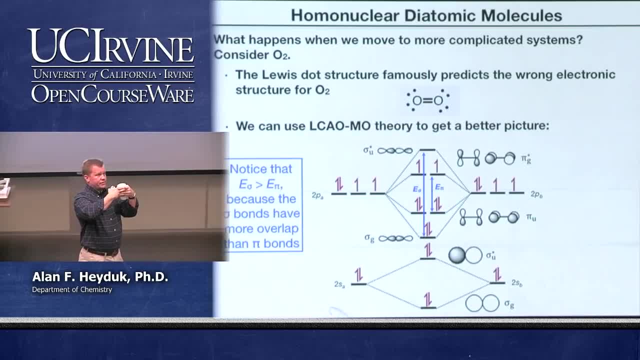 which are pointing directly at each other is better than the overlap between two pi orbitals that are kind of coming up. they're pointing parallel to one another and cozying up next to each other. OK, When we have this diagram, you can write electron. 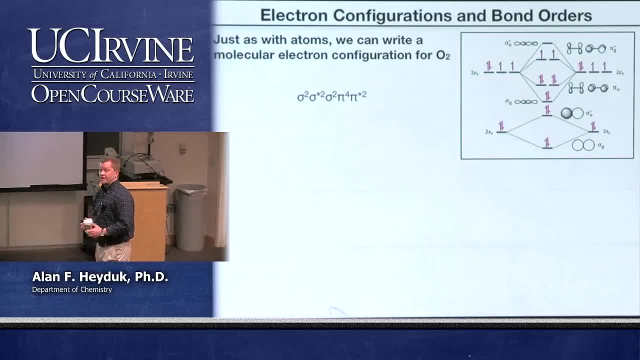 molecular orbital electron configurations. Remember how much fun you had with this in freshman chemistry. You know 3D, 6, you know blah, blah, blah. Well, we can do the same thing and have just as much fun with molecules. 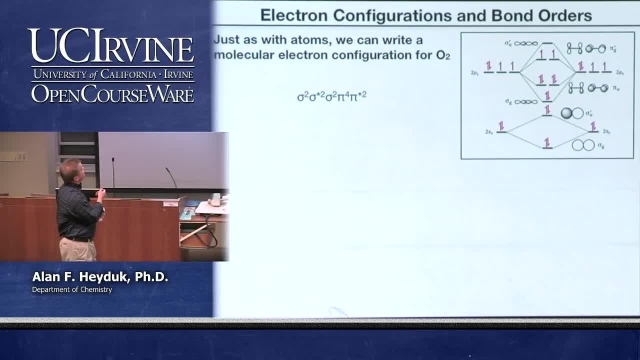 In this case we would write it as sigma 2, sigma star 2, that's the sigma from the S and the sigma star from the S. Sigma 2, pi 4, pi star 2, we have that filled sigma. 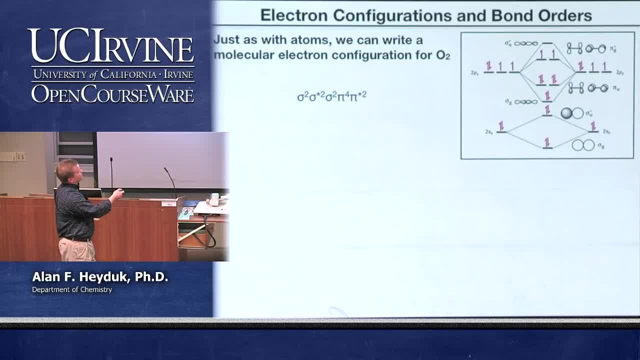 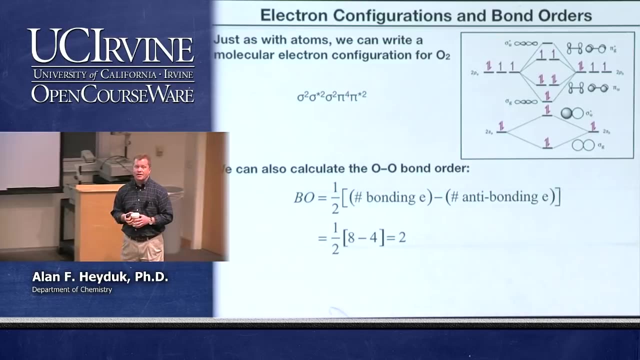 from the PZs, the filled pi from the PX and PY and the half-filled pi star from the PX and the PY. So that's our molecular orbital electron configuration. We can also calculate the bond order. This is universal for any isolated bond. 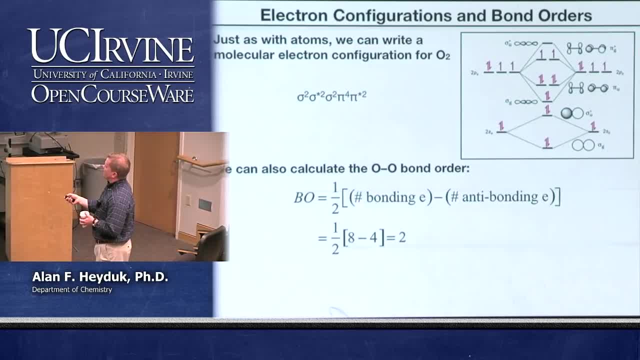 OK, We can calculate the bond order as the number of bonding electrons minus the number of anti-bonding electrons, all divided by a half. So if we just look at this diagram, we have two electrons there in a bonding orbital, two here in a bonding orbital and four there in pi. 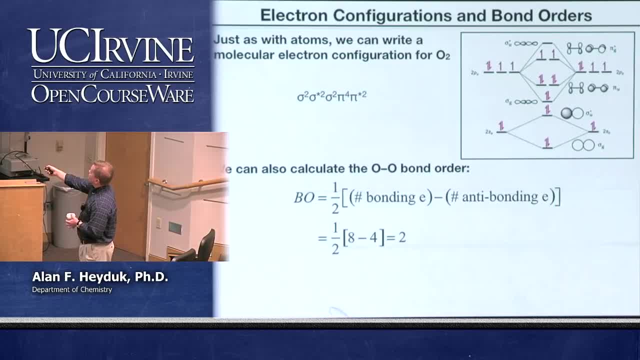 so that's a total of eight. We have two orbitals in this sigma star that comes from the S orbitals and two electrons in this pi star. that's four. so one-half times eight minus four is two. We calculate that the bond order for O2 is exactly two. 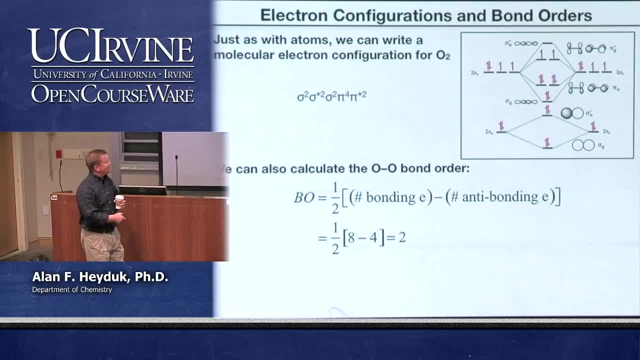 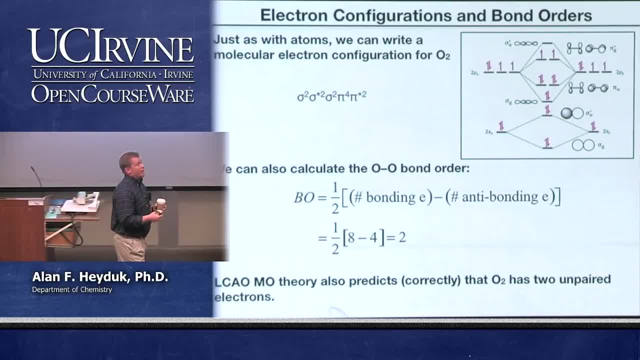 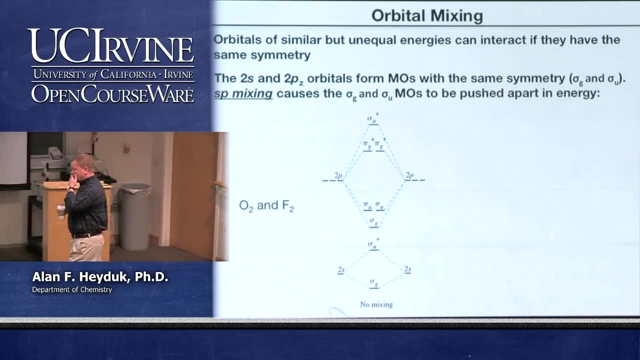 All right. So MO theory is great. It's wonderful Way better than hybridization and all that stuff that you learned in organic chemistry. We won't talk about all the problems that MO theory has yet. We'll get to them. So you know, we all know what really kind of sucks. 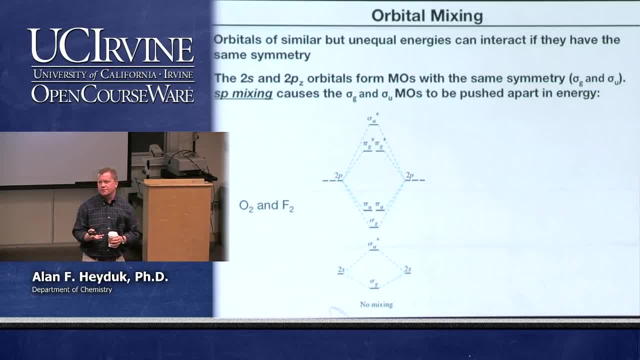 about chemistry. right, It started in freshman chemistry. It started in freshman chemistry. You would be told, kind of given out this simple model, This is how it all works. You're like, okay, I can remember that. And then the other shoe drops. 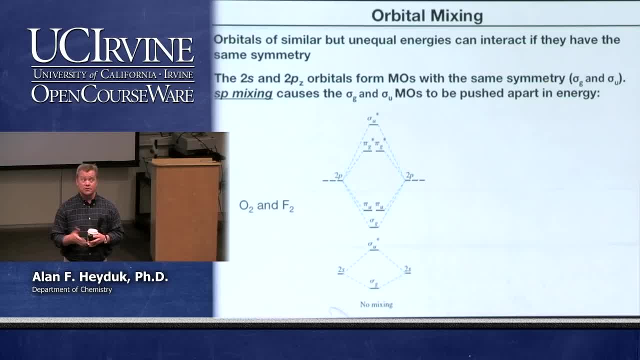 And you find out. well, you know, the model mostly works, except when it doesn't and you have to make this other approximation. And then you're like: okay, I can remember that one and then another one, you know. 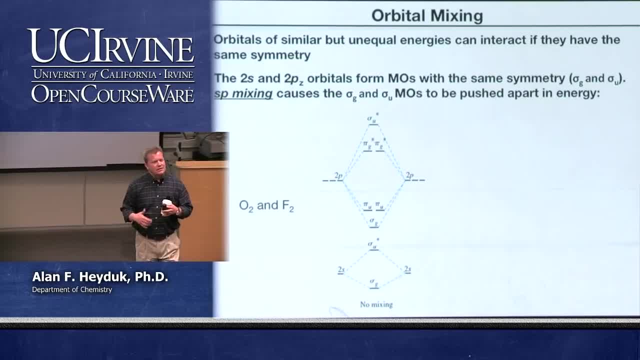 And so it just. we just keep piling on these things where you have to make your simple model more and more complicated to reflect the real data that we collect in the lab. So here's your first one. Here's another representation of that MO diagram. 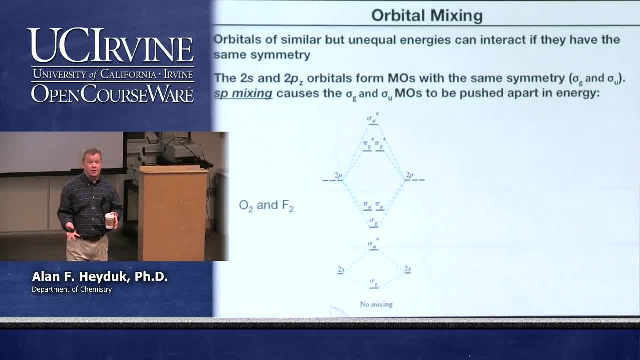 that we just drew for O2.. If somebody asks you to draw the MO diagram for fluorine F2, you can use the same one. Perfect Works, great. If you look on the periodic table right here, that's going to the right. 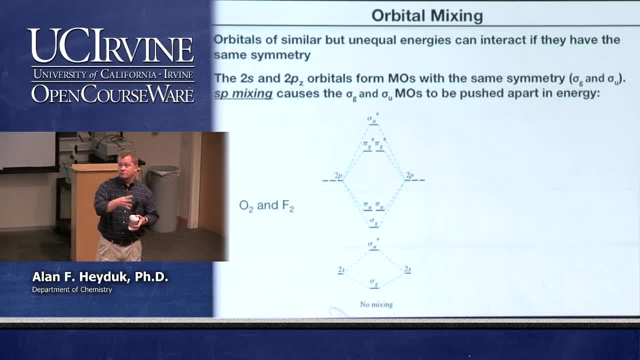 If you start from oxygen and go to the left. okay, what element? You guys are all juniors and seniors, chemistry majors at UC Irvine- To the left of oxygen, Nitrogen, Nitrogen. okay, Boy, I didn't memorize the periodic table either. 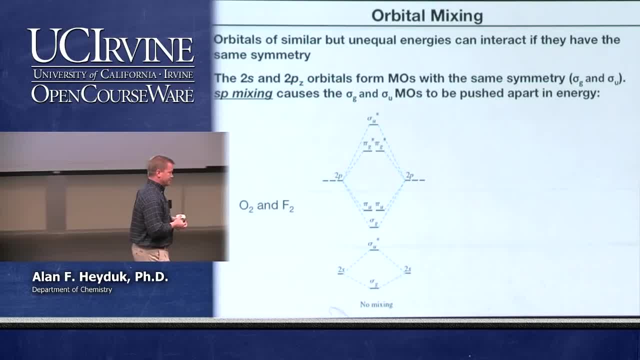 That's. I figured that's what it's there for. Okay, So we go. what if it happens? if we start at oxygen and we go one to the left? We just are basically taking one electron away from each atom and making the N2 molecule. 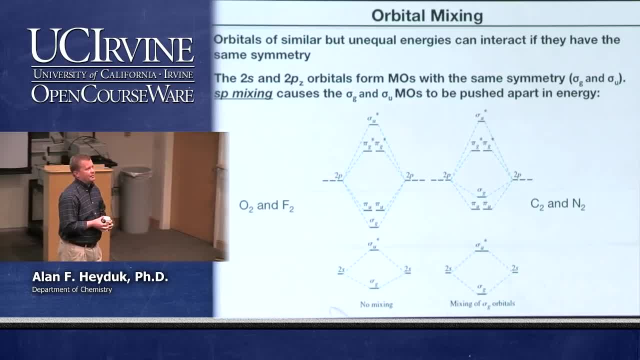 So there's the MO diagram for that homonuclear diatomic. If you have really bad eyesight, it probably looks the same to you. If you don't have bad eyesight, you'll notice that somebody screwed up the ordering of those orbitals. 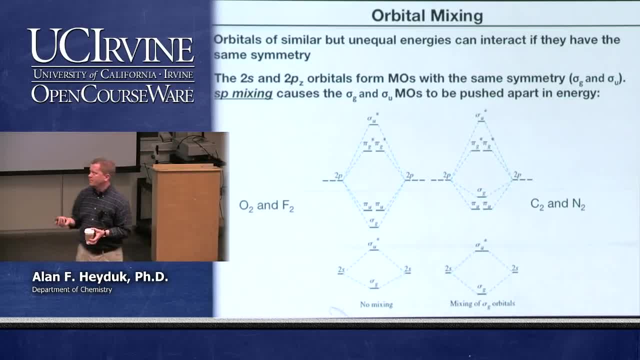 Synthetic, Synthetic. Since when is a sigma bond weaker than a pi bond? I know all of you organic chemists are out there saying, yeah see, look, your model sucks too. So the question is: what's going on, And did we just draw this incorrectly? 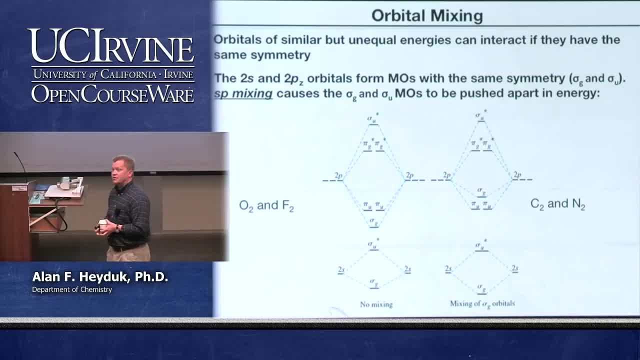 The answer is no. We drew it this way first and then realized, when we went and did experiments, that the model didn't fit the data. So we had to refine the model. And then we had to wave our hands and come up with an explanation why we were refining the model. 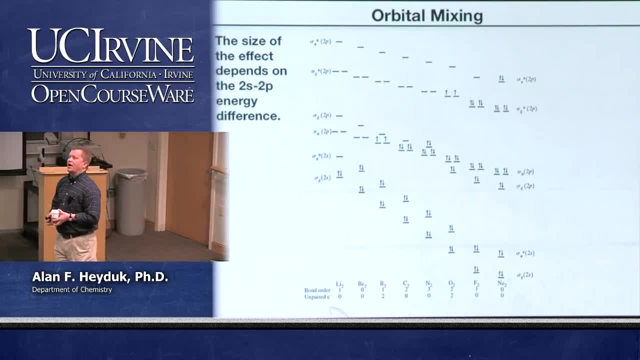 So what's the explanation? So here, there's a lot of data on this slide, okay, All we're looking at, and it's all really small, so I hope you got the notes last night. We're going from dilithium to diborane. 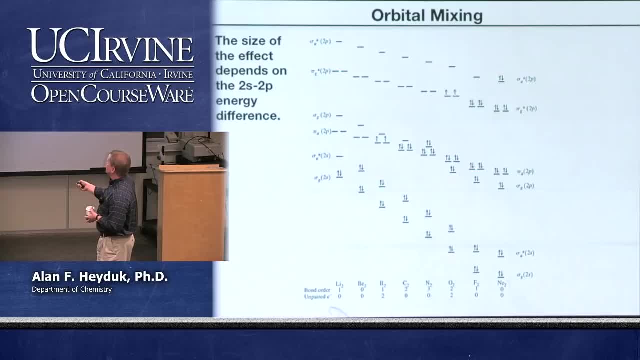 To diberyllium, diboron, dicarbon, dinitrogen, dioxygen, difluorine and dineon. okay, Right across the second row of the periodic table, And so, if you look carefully, we're just going to focus here. 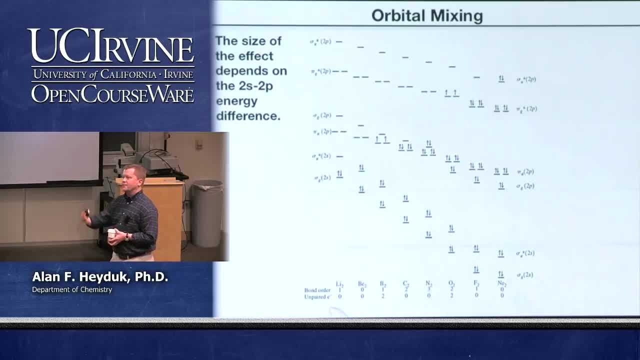 for now on the sigma and pi orbitals that come from the combination of two p orbitals. And you see, for lithium, beryllium, boron, carbon and nitrogen, all of those have this situation Where, for some reason, the sigma orbital is higher in energy. 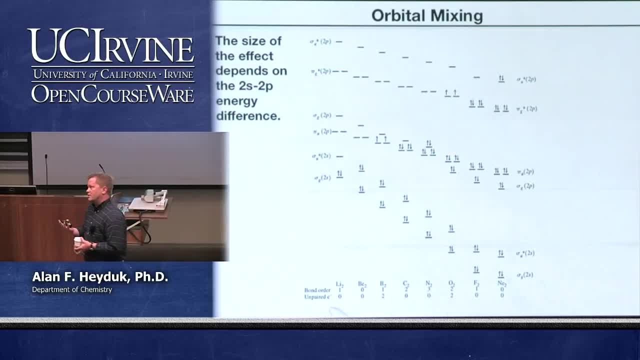 than the pi, which is another way of almost saying that the sigma bond is weaker than the pi bonds, Which again, we know from organic chemistry, makes no sense whatsoever. Once we get to oxygen, the order corrects itself And the sigma is lower than the pi. 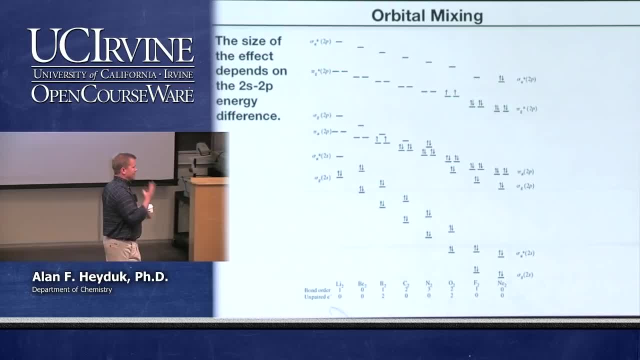 For oxygen, fluorine and dineon, even though dineon doesn't really hold together. Okay, so what could be causing the problem here? It turns out that the information is right on this slide. I only wanted to ask. so this is the energy based. 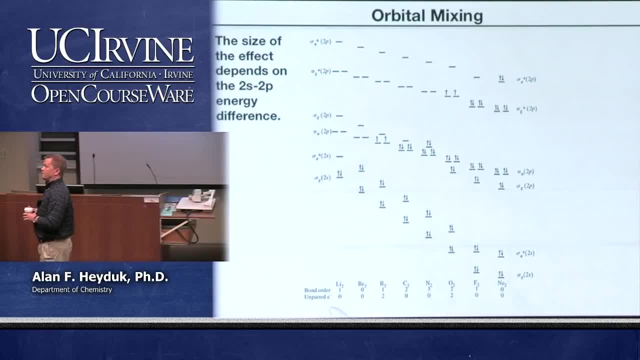 on the model and not on experiments, right? Yes and no, Yeah, okay, So, So it's so. it is the energy. it's the diagram from the model that is modified to fit the experimental data. okay, So, so these are the correct electron configurations based. 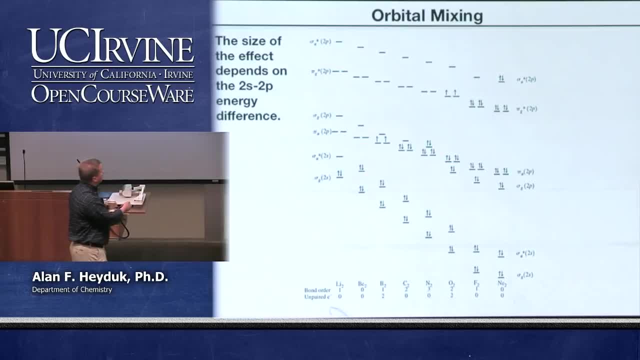 on experimental data, But again the model's been tweaked. you get this crossover between if the sigma's lower or the pi's lower, Okay, so that's a good, that's a really good observation. Oxygen is the first combination that has electrons in the pi star. 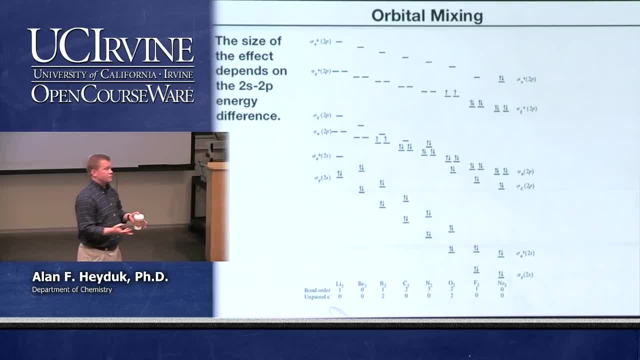 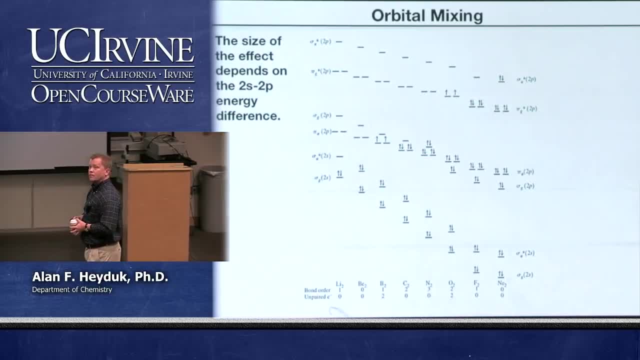 But that's a really good observation. good eye, You'll notice there's something else changing as you go from left to right across this table. Electronegativity is changing. And so what's electronegativity It's? it's how tightly the nucleus holds. 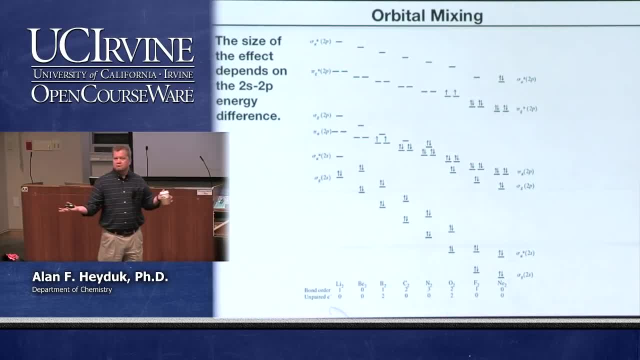 on to the valence electrons. That's a fair description, right? Okay, when in in molecular orbital speak or atomic orbital speak, that means the orbitals are lower in energy. Oh, you're just looking ahead on the notes, aren't you? 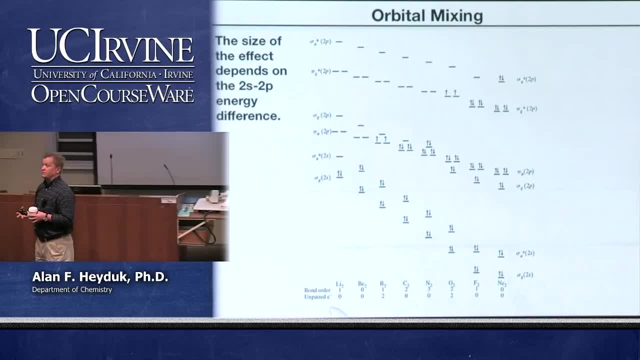 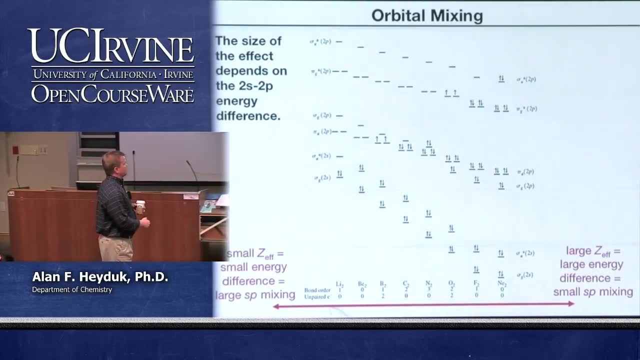 So effective nuclear charge Z effective is what? one of the factors that controls electronegativity? Okay, But look as we're going across. look at what's happening to the sigma orbitals, the sigma and sigma star that we derive from the S's. 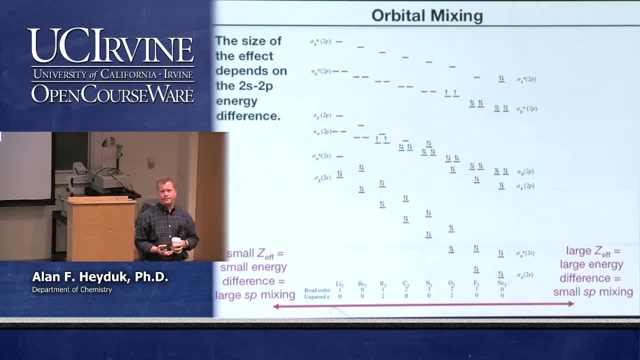 They're dropping like a rock And so these are all tied together, right, Remember S orbitals. There's in a for an S. right, there's the two of them orbital. there's actually a probability that the electron could be at the 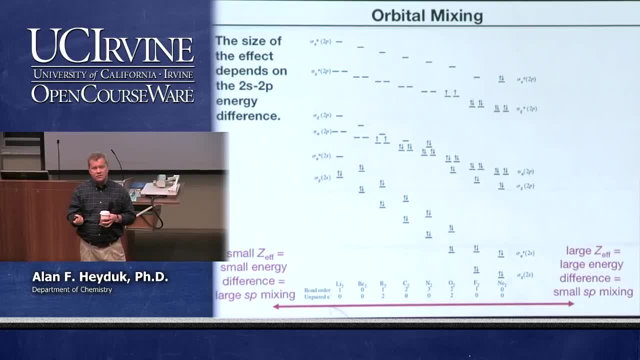 nucleus. So what that means is that s orbitals really feel the effects of an increase in Z effective. It affects s orbitals more than it affects any other type of orbital, because the s orbital has electron density at the nucleus. The p, remember, has a node. There's zero probability of an electron in a p. 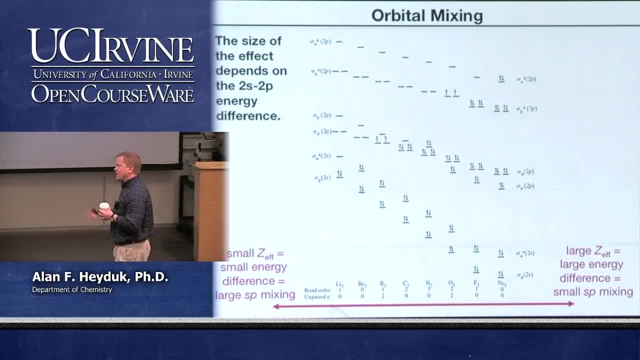 orbital being at the nucleus, So it has less of an influence. These are dropping like a rock, Okay, so this is where things get a little screwy, or it's going to seem like they get a little screwy. See that symmetry label there. We said that the bonding combination between the 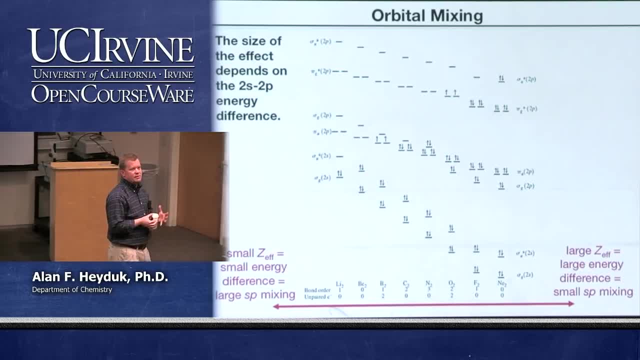 two s orbitals, that sigma bond. we ascribed a symmetry label of sigma g to it. The sigma orbital that comes from the combination of the p z's also is sigma g. So remember what these symmetry labels are. It's the irreducible representation. So these 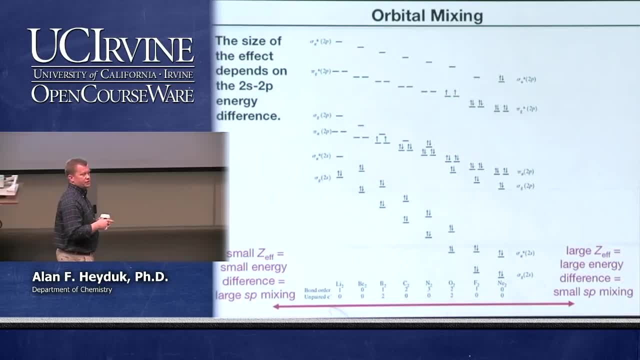 two sigma orbitals have the exact same symmetry, They belong to the same irreducible representation. We said that if we have two orbitals of the same symmetry, they can interact, they can mix. That's what's going on. Remember, we also said that the strength of that mixing 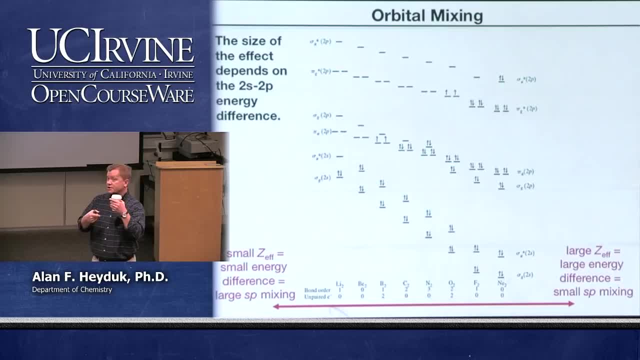 is inversely proportional to the energy separation. That is, when the energy separation is small, the mixing is significant. When the energy separation is large, the mixing is significant, and if the energy separation is more than equal to the energy you're matching with. 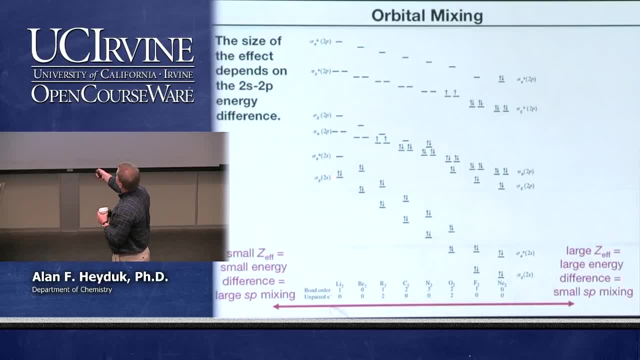 Mixing is insignificant Here. the energy is pretty small. So what literally happens is because this sigma bond is the same energy as this sigma bond, you can think of it as they repel each other. This one is actually pushed down a little bit more than it normally would be. 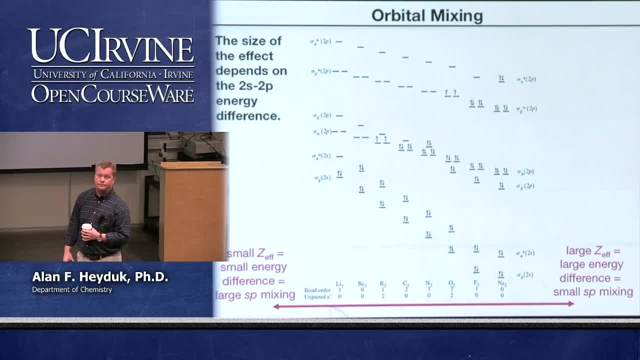 This one gets pushed up higher than it normally would be. Same thing here, same thing here, same thing here. What happens when we get to oxygen? Well, we've gone over the threshold. This sigma G combination is just too far away to interact significantly with that sigma. 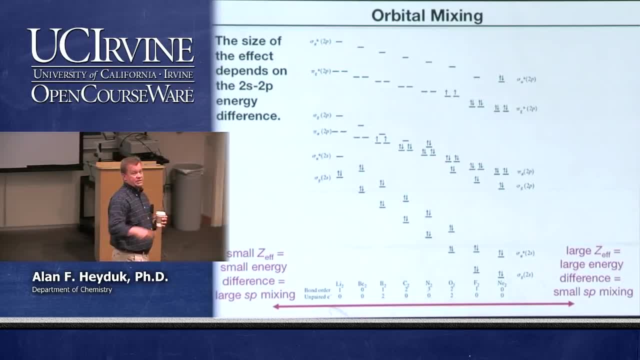 G, And so this one does not get pushed down, Pushed up above the pi. So we call this configuration interaction, Or you can use another term that we've all used improperly before hybridization. This is what I like to say: it's hybridization done correctly. 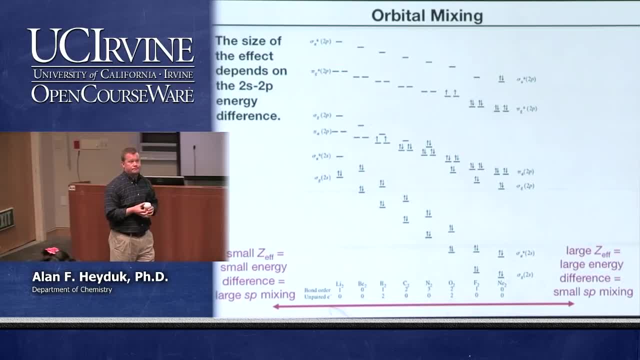 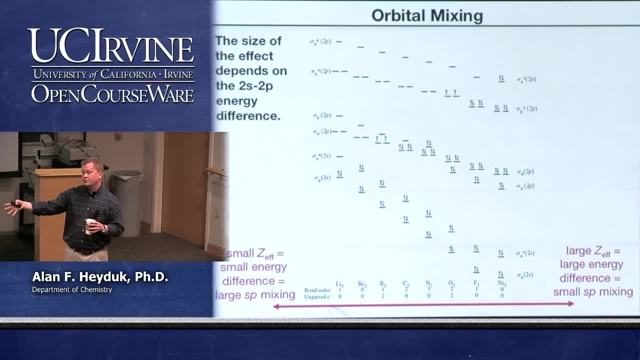 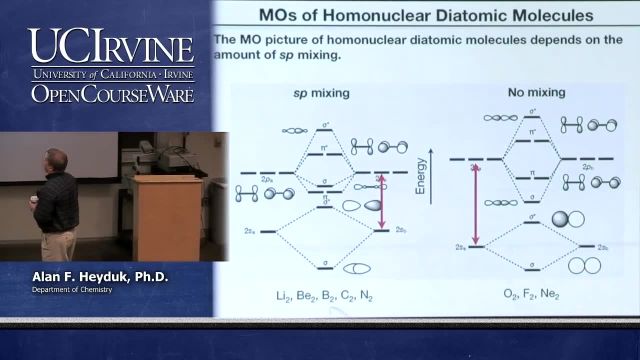 to get the simple model to reproduce experimental data. We're gonna see all kinds of examples where this happens, But for our purposes, if you're asked for the diatomic MO diagram for lithium, beryllium, boron, carbon or nitrogen, 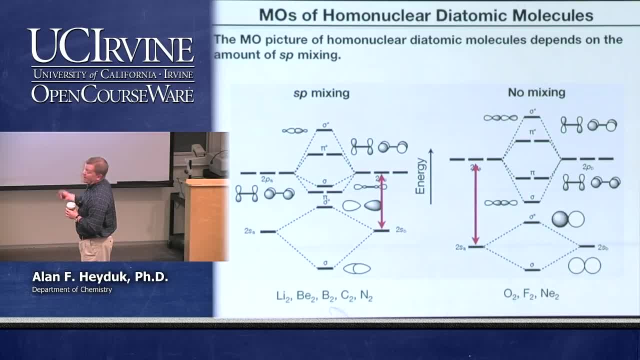 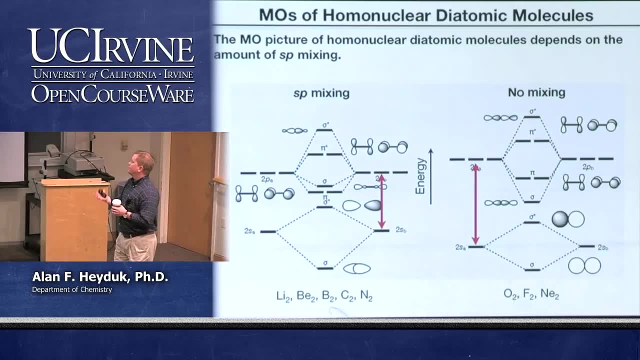 just remember that sigma is above pi. If you're asked for oxygen, fluorine or neon, you get the traditional ordering where sigma is below pi. Now some of you that are thinking ahead are like: well, okay, what happens if we do the CO molecule? 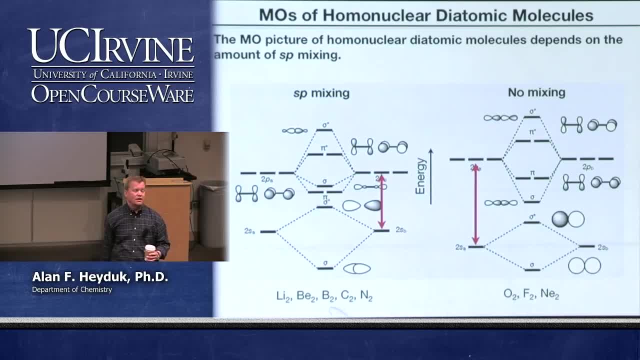 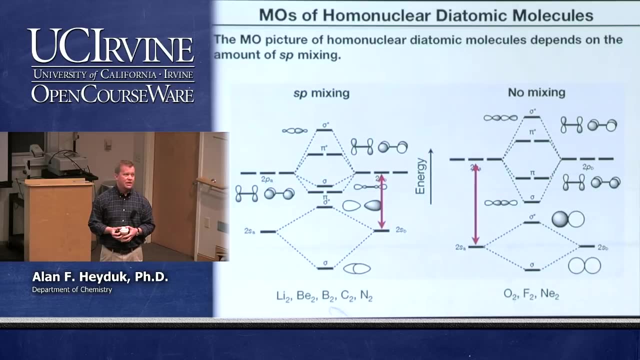 We have one from this side and one from that side of the line, Without any added data. always assume this traditional ordering, In other words, that your sigma bonds are stronger than your pi. If you're given some other data, the compound is this number of unpaired spins. 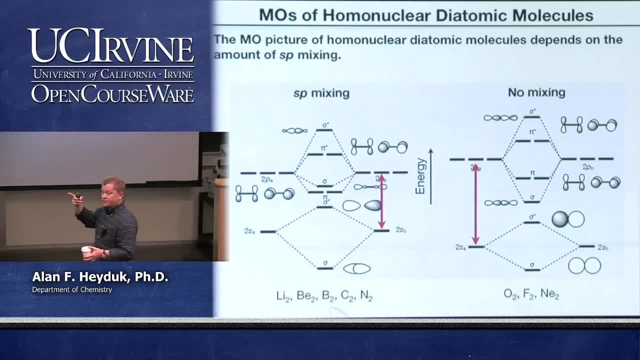 where you have to flip the order of orbitals to get the right number of unpaired spins, then you can apply this kind of fudge factor, And so that's what happens with all of these situations where the model breaks down, And I know, as students, you worry about this. 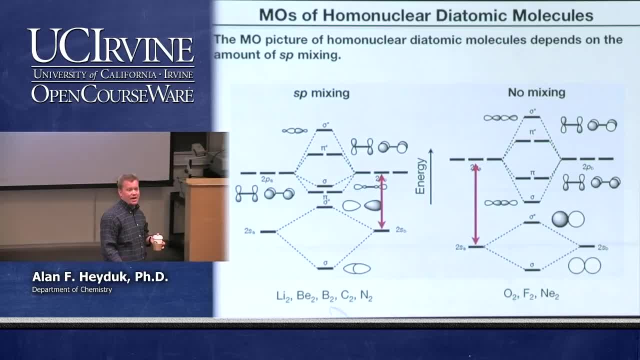 because you're like: well, what if I'm asked a question on a test and it's one of these weird ones where the model breaks down? Well, the only way that we get it right is to go make a measurement and get a piece of data and realize we have to fudge the model. 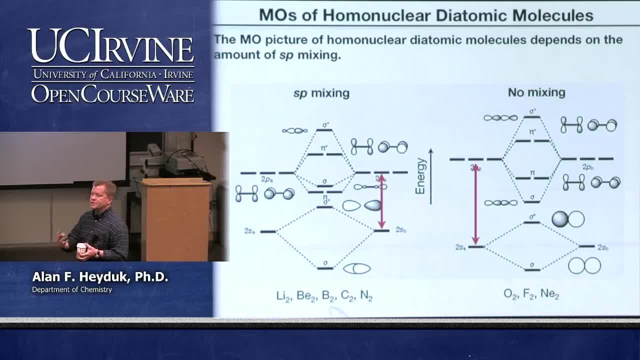 Or improve the model. So it's the same thing for you. This is a case where I'm already telling you. if I ask on the test for you to do the diagram for diboron, you have to remember that it's on the left side of the line.